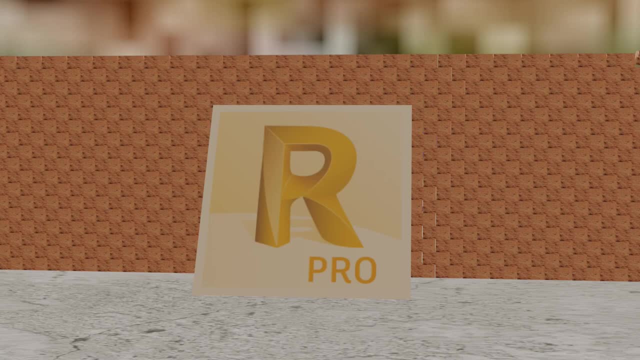 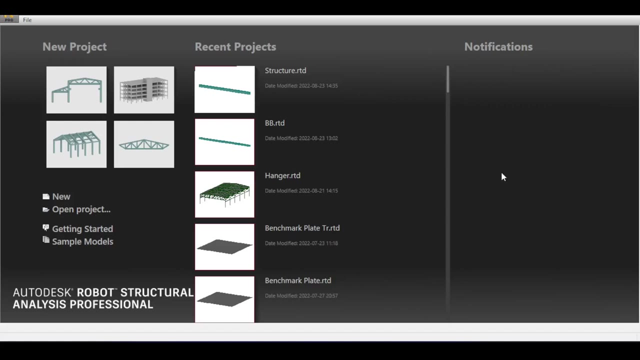 Hello everyone and welcome to the Autodesk Robot structural analysis tutorial brought to you by the Civil Engineering Essentials channel. I hope you enjoy the video. In this video we are going to discuss how Autodesk Robot calculates the provided reinforcement for beams. So to start with, 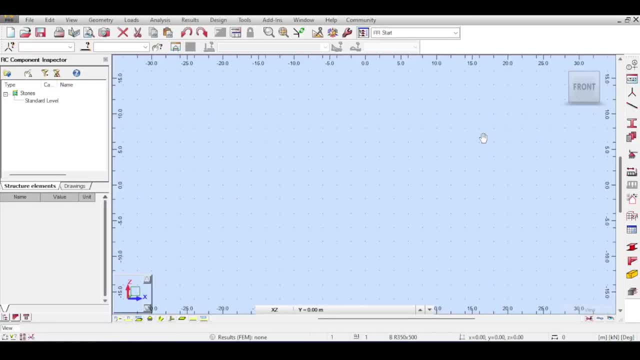 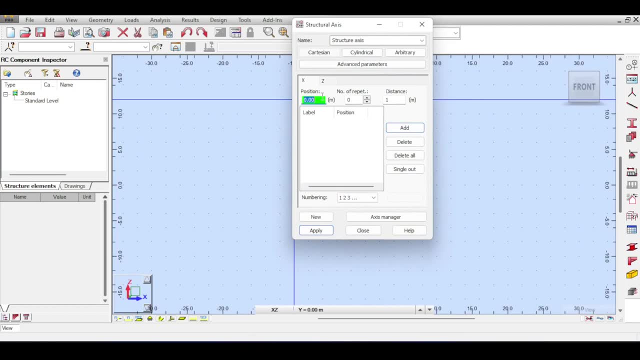 I'm going to select my 2D frame design. Now I am in my 2D frame design GUI. Of course, this environment has been explained before in a video about understanding the GUI of Autodesk Robot. Please feel free to check this out. So I have my beam and my beam is going to be a two span beam. 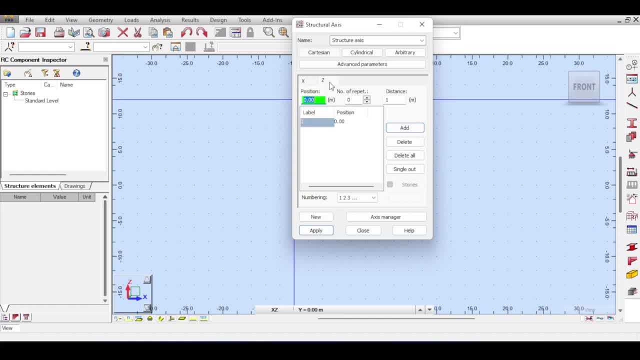 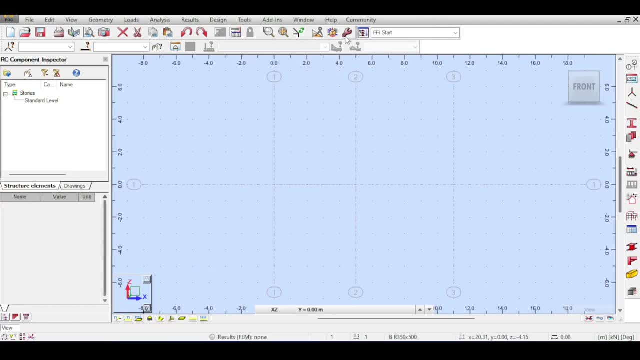 The first span is five meters, The second span is six meters, And well, I'm just going to define me a beam Before I start. however, since I'm going to design stuff, it's worth it to mention that I'm going to design my structure using the ACI code, So I'm just going to click on the wrench. 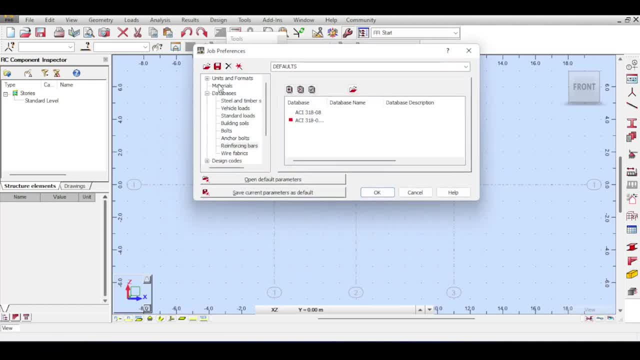 tool, go to my job preferences and double check that. Of course, checking job preferences was explained before in yet another video that is once again linked above, But I'll just quickly go through it very fast. So for my materials I'm going to use American. 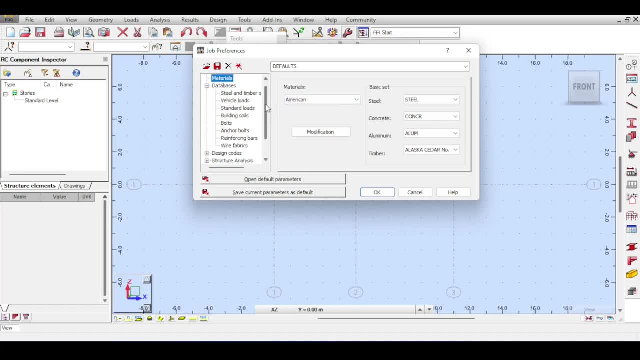 materials because I'm designing using the ACI code is the American code. Feel free to add any material or change that data base according to your design code. I'm designing using the ACI code, So my materials are going to be American. For the design code, I'm designing using ACI 318 metric. 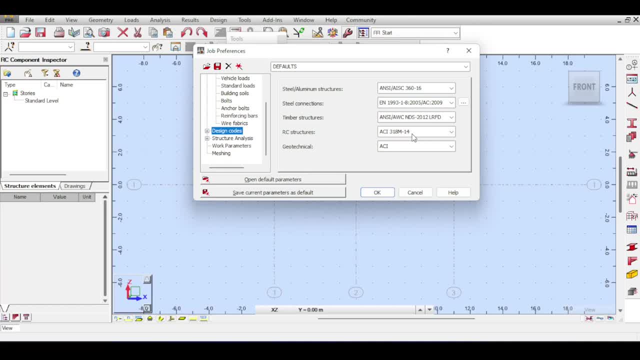 and this is the latest design code in Autodesk Robot for the ACI. Maybe in the future They will add the two thousand and eighteen addition For little airplanes. each one will have an éerstones material in them and each one will get a colors for normal aircraft. 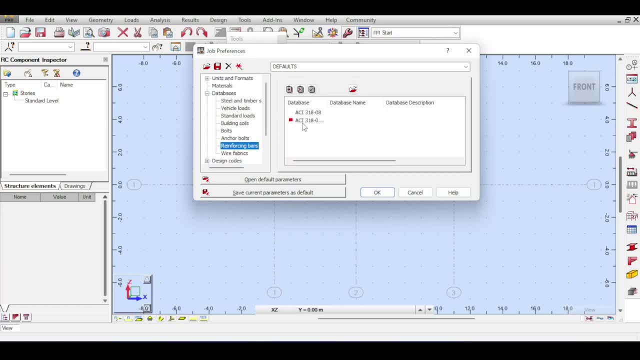 databases. there is something called steel reinforcing bars and i'll make sure that i'm selecting the metric and clicking the current database here, because i'm a metric guy and i want to design my reinforcement according to the metric reinforcing bars, the difference being that in the metric the bars are named by their diameters, whereas in the imperial, or diameters, have numbers, 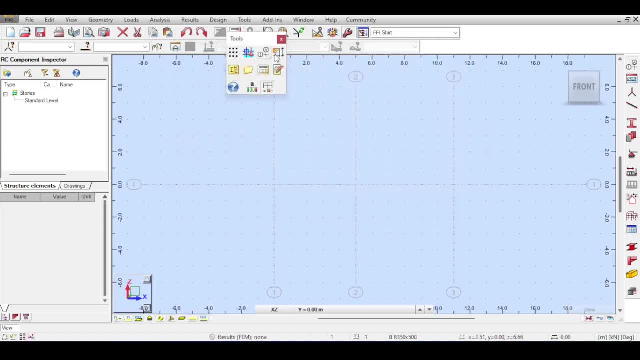 so right, everything seems to be nice, so just click ok and start modeling my beam. of course, modeling the beam was covered in a previous tutorial for me. i'm going to model a reinforced complete beam with a cross-section of 350 by 500. the cross-section was chosen according to the aci. 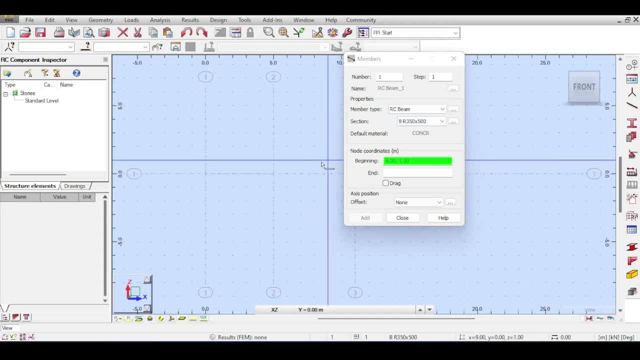 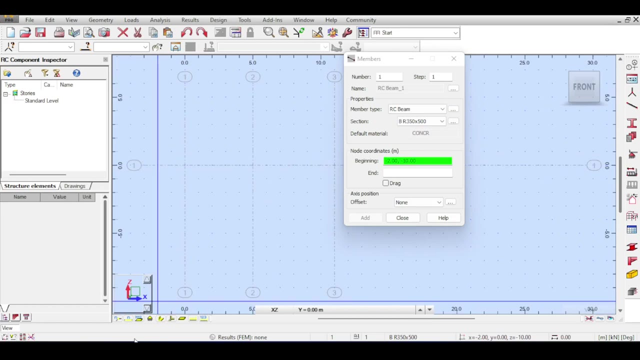 code. the aci code states that you can skip the deflection calculations if you choose a beam that has a height which is stipulated in the aci code. in my case, my two spans are one end continuous and my height should be of the beam should be l over 80. 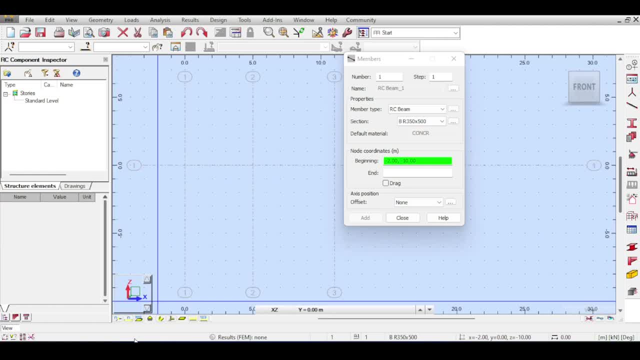 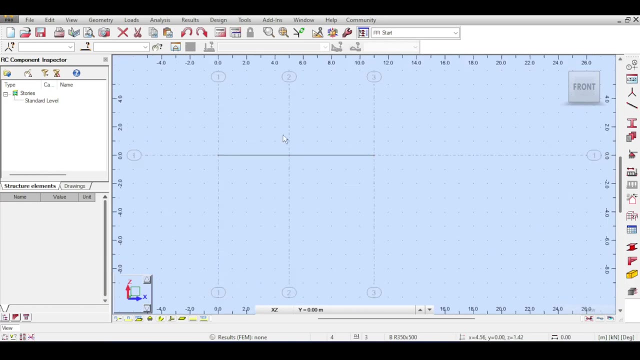 point five: six meters over 18.5 is less than 500 millimeters, so i'm more than satisfied with this and this beam should satisfy my deflection control, which means i don't need to control my deflection for this beam because i'm following the aci code suggestion. all right, so i have my beam now. i'll. 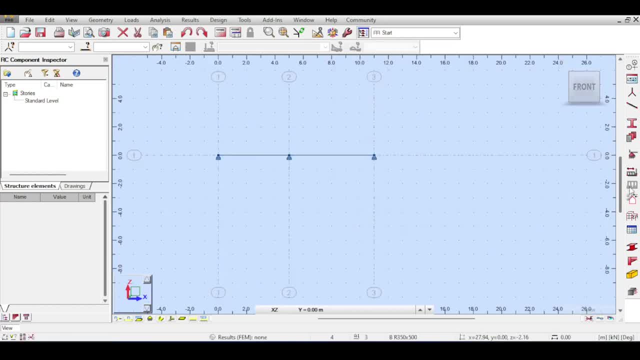 just support it very quickly. i'll add me some pin supports and i'll add me two load cases: one dead, which will include the dead load, and one live, which will include the live load. the dead load has pre-calculated in it the self weight. you can double check this using the table. this was also. 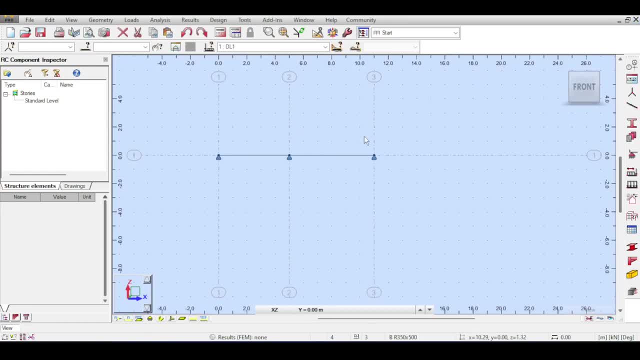 explained in the previous video is going to be linked above all right. so for my dead load, i'm assuming that my load per unit area is 10 kilonewtons per meter square and that the beam has a tributary width of five meters, which means that in the dead load my beam is going to have a 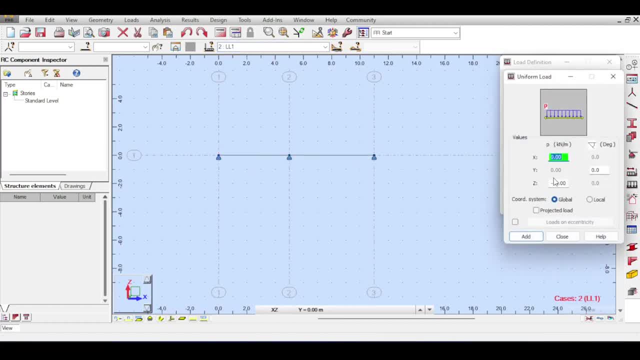 50 kilonewton per meter dead load in the live load. i'm assuming a three kilonewton per meter square live load on the plate. so my beam is going to have 15 because it has a tributary width of five. fantastic, so if 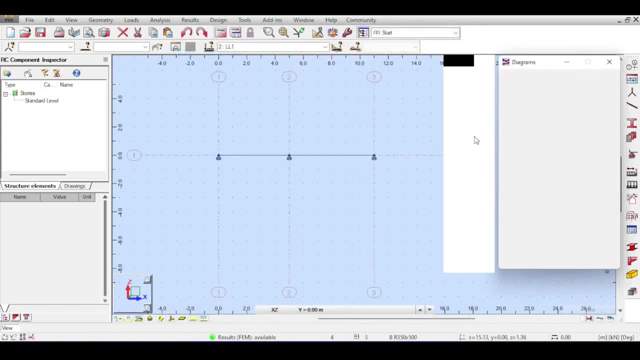 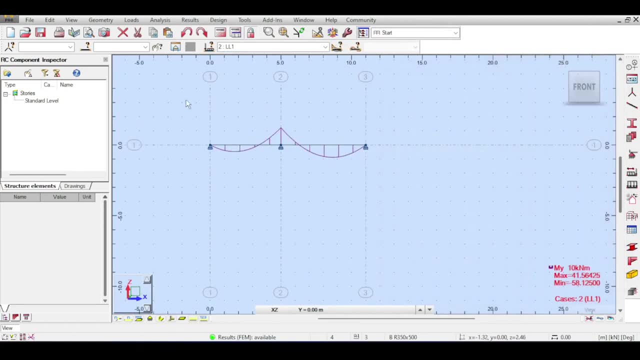 i run the analysis now. quickly go to results diagrams for members. check mi. click. ok, you can see i have any moment diagram. i have nothing wrong, so everything seems to be fine, fantastic. so let's take this beam and click on design. now i have explained required reinforcements in the video. 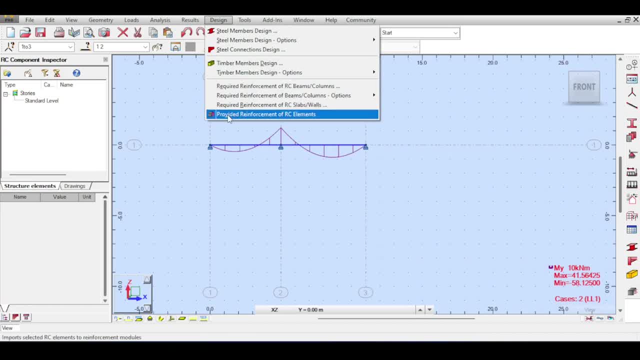 before, which is once again linked above, but for today i'm going to check the provided reinforcement. that here, robot calculates the adsd required and you are responsible for distributing this adsd required. and the other option: robot distributes reinforcement for you, which will take a little bit more details. i click on that now. robot will start importing the structure. 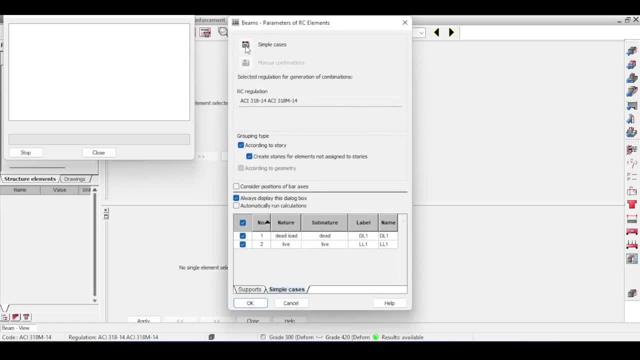 you can import the loads based on the combinations or in simple cases. i am using simple cases because i want robot to perform the combinations for me as well as perform the load. the live load case of floating, meaning that it is going to variate the live load on all the spans. all right, fantastic. so 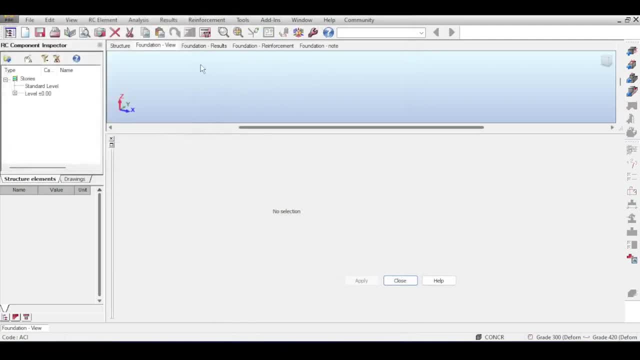 i have it right now. i just once again click on: okay, so now i am in my design view. now i have imported my beam as well as my foundation, because it seems a little bit thought that my pins are actually foundation. i'm going to talk about my beams today, so i'll double click on my beam, which 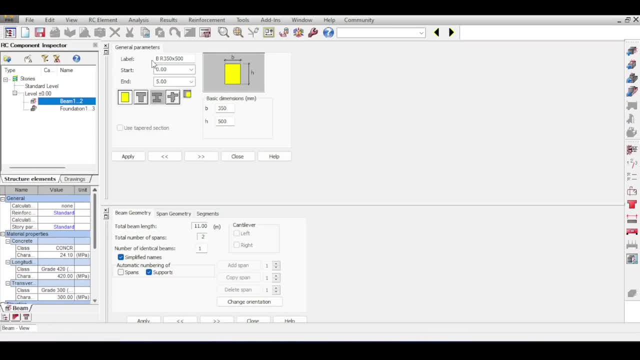 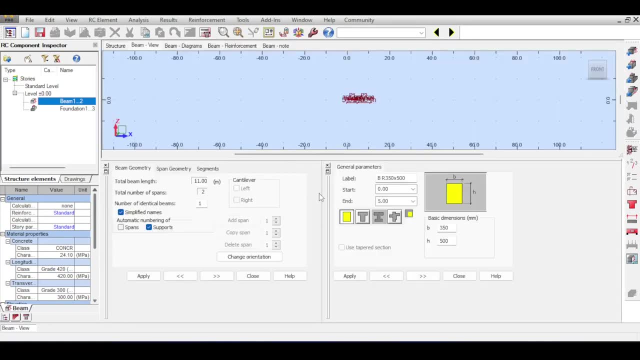 opens the beam design gui. and i have, it seems i have a problem that i don't see my beam. now, if you have the same problem, you click on this little window button and drag this to the side and now you can see everything, because now you can see your beam and you can see your inputs. now you are. 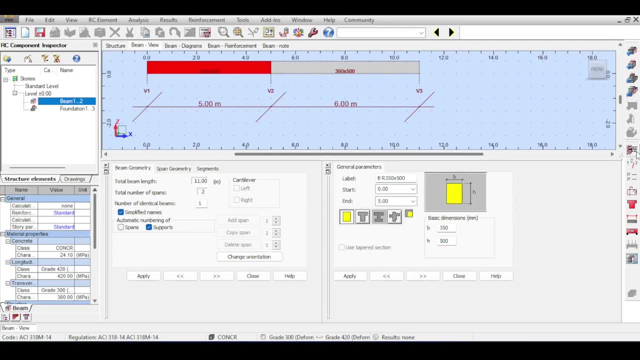 in the input section of your design. you can see that there are multiple options here. those options are with regard to your beam and we are now in the input and the geometry input of my beam. now, first of all, my span geometry has a lift support and now we need an assumption. i'm assuming that 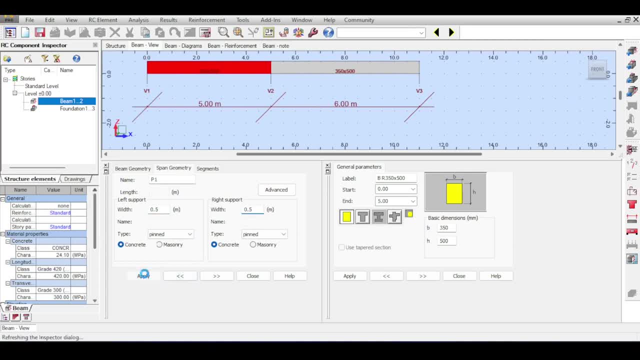 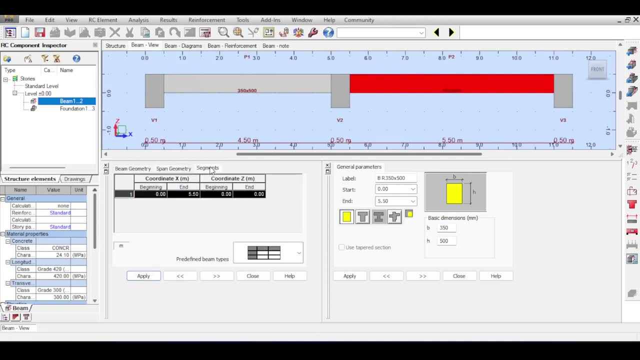 my column has a width of 50 or 0.5 meters. you plane of the beam, so i just do that very quickly. all right, fantastic. now there are some more things for segment, if you want to change stuff, like if you want to have a beam that is inclined, or 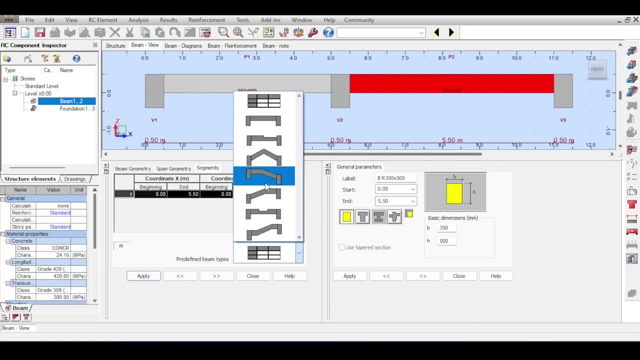 something. you can use this for staircases if you want, especially this one. i will not do anything because here this is only an introductory video. i will talk about staircase design later, but for now i just keep it as simple as possible, because there is a lot of stuff to be covered, all right, so. 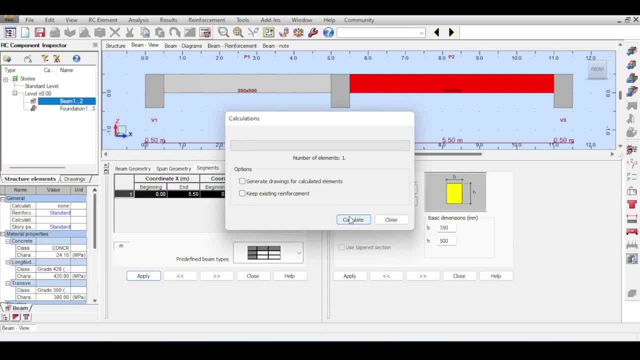 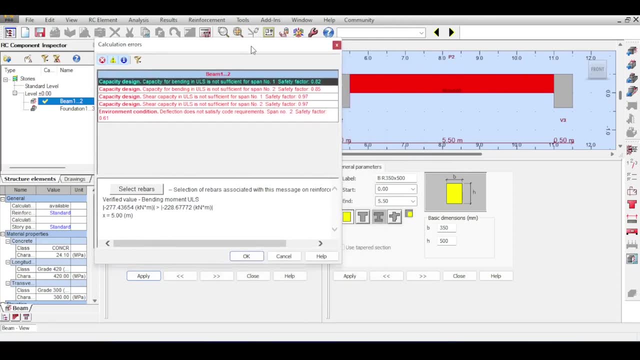 now, if you do a quick blind calculation, everything is not going to work. let's take a look: you will be bombarded with millions of millions of arrows, which will basically, first of all, put you off. but let's well, let's dissect those arrows one by one. you see, you have four arrows related. 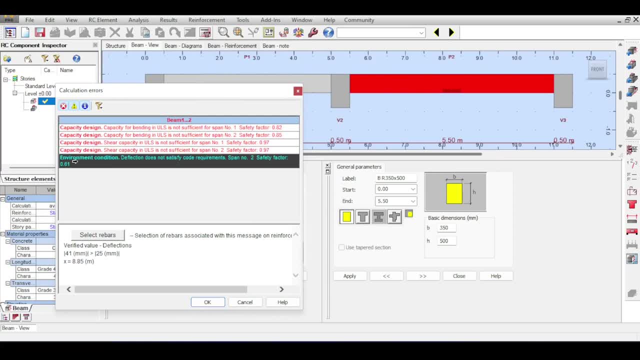 to the design capacity and one error related to the environmental conditions or the service limit state. and well, first good news is that the deflection does not satisfy code requirements. nobody cares about this, because we have assumed the height of the section conforming to the acai code and, in that case, the acai code. 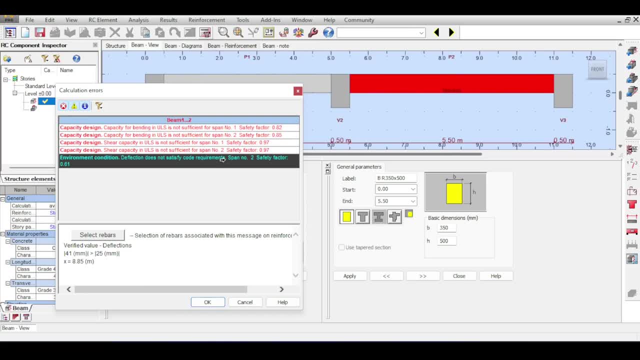 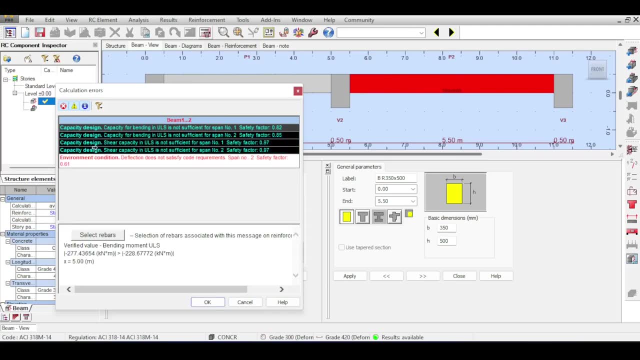 actually tells you that you need not check deflections because this height is satisfying and good. but well, i still have a lot of other problems and those are really dangerous. i have capacity and design problems, which means that the beam i have now is not able to hold or withstand. 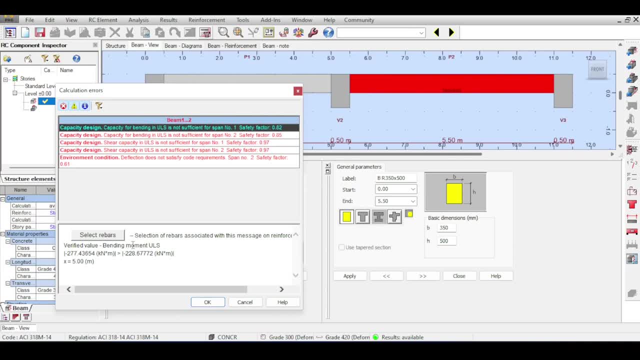 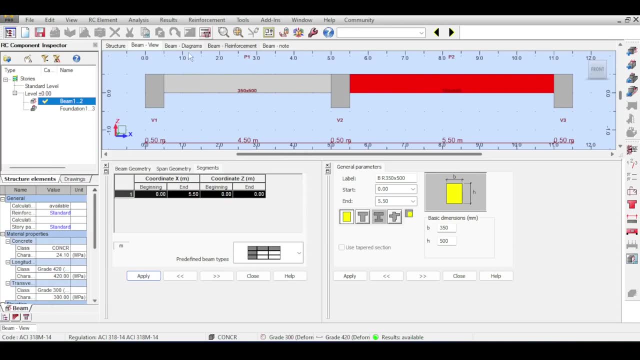 the forces applied. now, if you click on anyone, it tells you that, for example, the bending moment has a problem. now how do i see this? well, let's forget about the error for a second and look at something called beam diagrams. if you click on that, you see the. 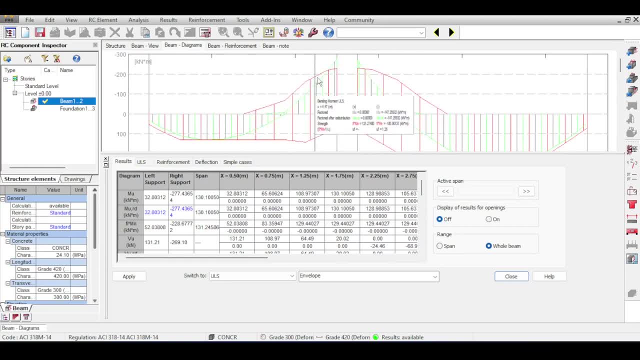 bending mode. diagram of the beam. now, the green line here is the applied bending moment on the beam, whereas the red, whereas the red here is the ability of the beam to resist, and you can see that near the support, the green is larger than the red, which means that the applied forces are larger. 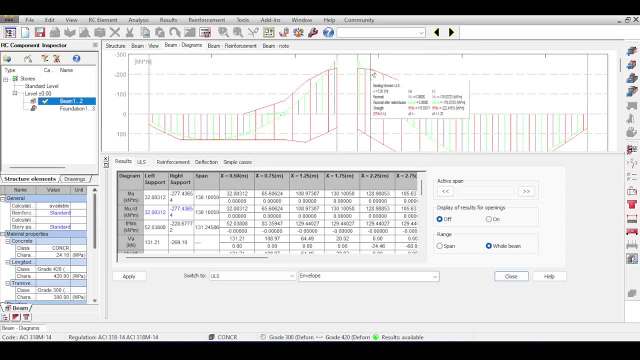 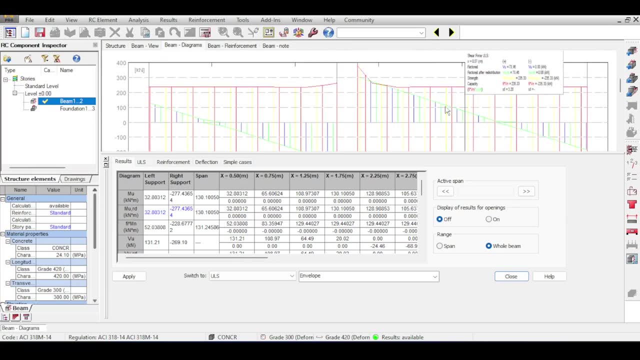 than what the beam can carry, and that's the reason why you get an error and the warning for this. so yeah, this is the first problem, and let's take a look on the shear. the shear seems to be fine. now there is a problem here. you can see, here green is more than red, which is basically a problem. 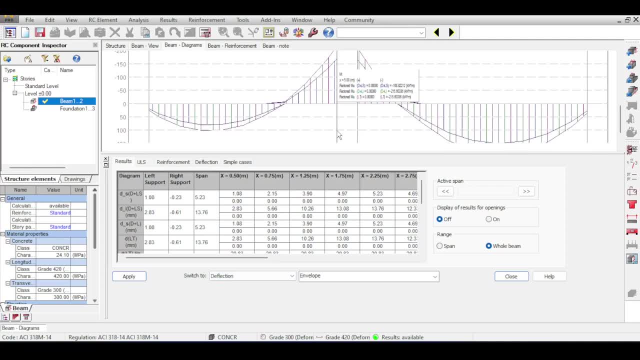 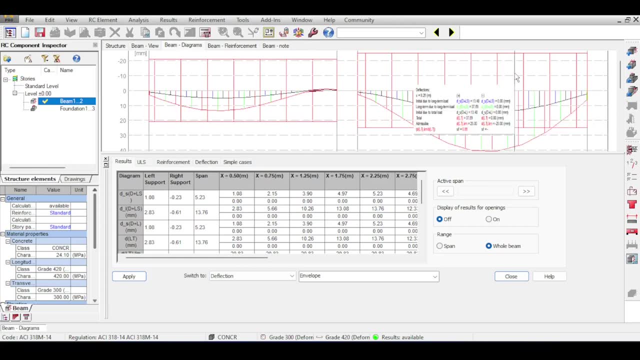 you can also switch from uls to deflection. and now you can see that, well, for the first span, deflection is satisfied. for the second span, deflection is not satisfied. the second span was six meters, so it's basically makes sense not to be satisfied now the limit of deflection that was. 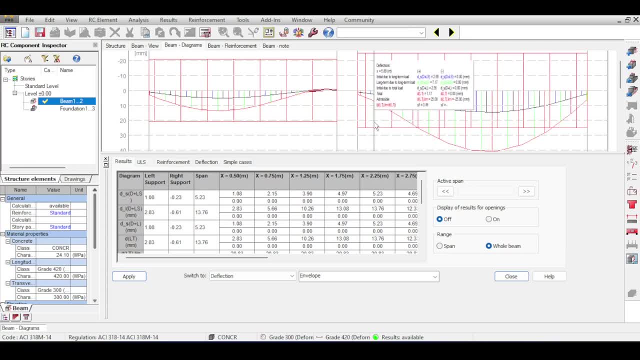 imposed here is a limited limit from autodesk robot, which is 25 millimeters. now, each code has its own limitation because usually the code limits the deflection according to a fraction of the span, for example l over 180, for example. i just leave it as is because for my deflection control i am abiding by the aci code. 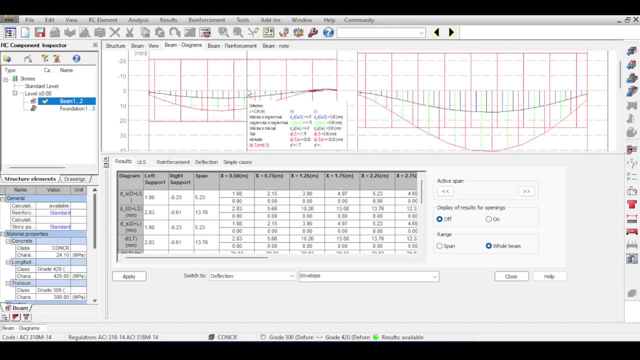 requirement that says if you are using l over 18.5 as a height for the beam, then you are on the safe side and you do not need to check the long-term deflections. and, by the way, this beam fails not for the short-term deflection. the black one is the short-term deflection. no, it fails in the 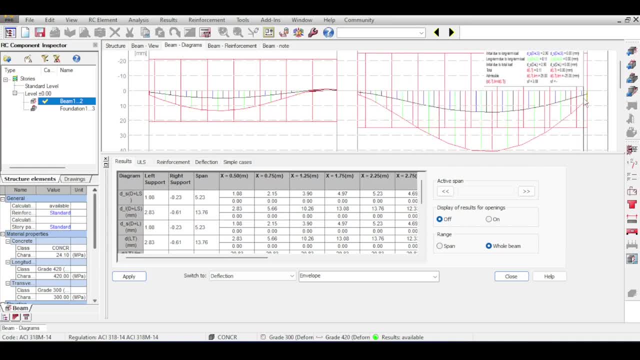 long-term deflection that actually includes creep and includes all kind of stuff, and please notice that for the long-term deflection different aci limitations apply rather than the short-term deflection, and you can check this out in the aci code, for example. it says that 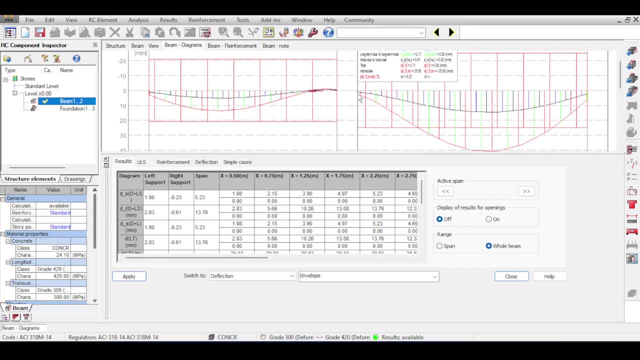 l over 240, i think, is what is the limitation for a beam if it's not holding anything that is deflection sensitive from live load only. so yeah, there is a lot of details to be covered here. i'm not going to cover this because i am abiding by the aci code recommendation. okay, so i have a problem. 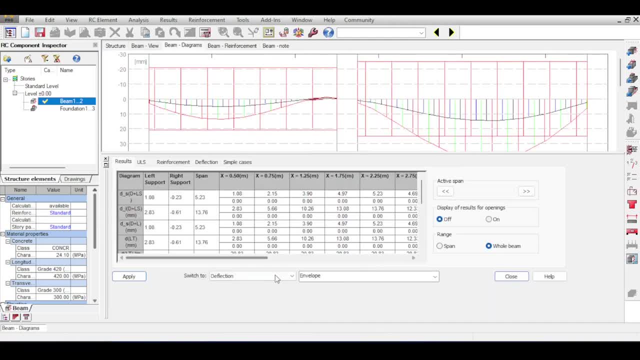 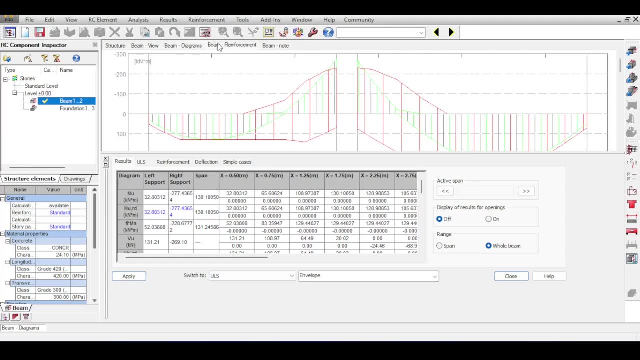 with my reinforcement, basically because it cannot carry it. you can see that if you go back to your uls, once again they have problem here. now why? what is actually the problem? the problem is that if you go to reinforcement you cannot see anything. so i'll just make this smaller and drag it here. 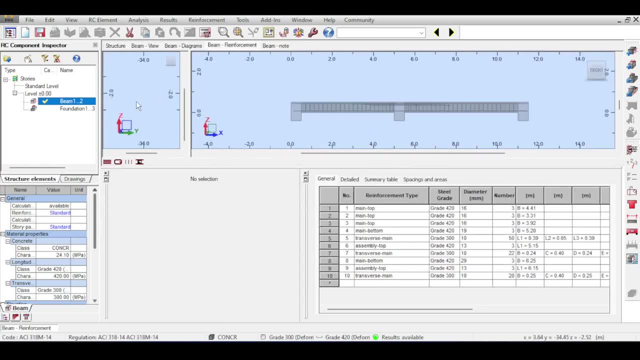 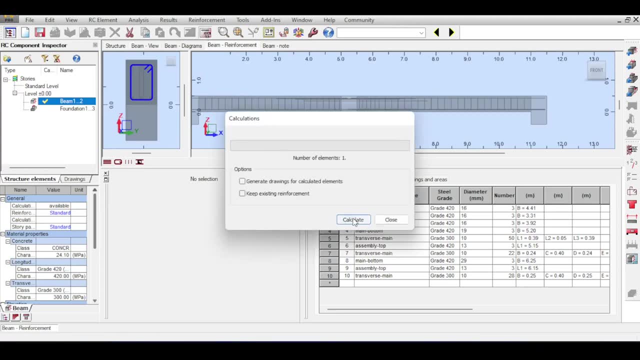 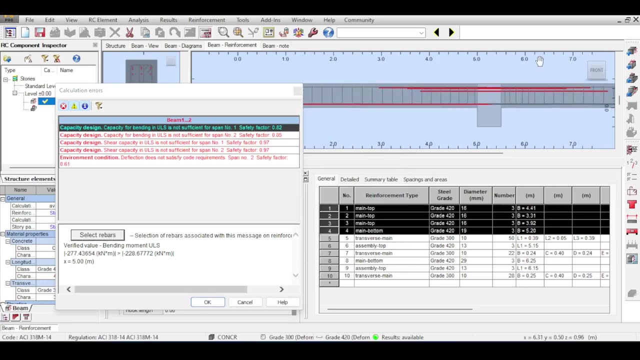 if you go to beam reinforcement and basically like zoom in just to see stuff, you can see that there is all kinds of strange reinforcement happening here and if you run the calculation again, it actually tells you where the steel is that has problems. so if you click, for example, on this, click on select rebars, it selects you the rebars that have problems. 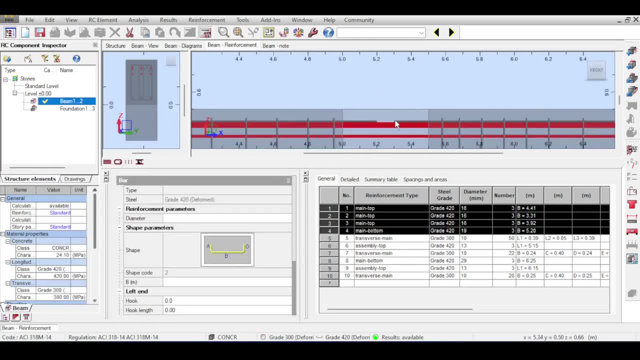 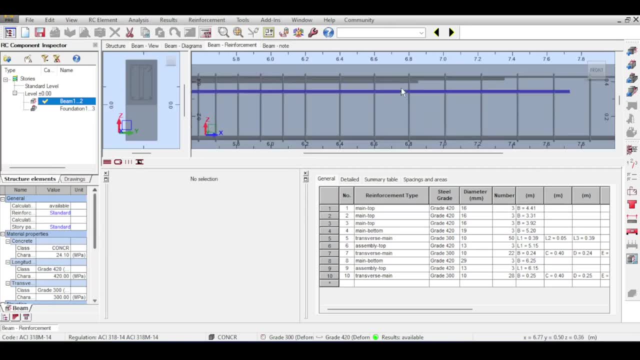 all right, so let's dissect this now. first of all, what is this? why is this not continuous? this is the first question. second question is: what are those steel bars? i mean, i see a lot of steel bars. this is not how like. this is not how my steel looks. 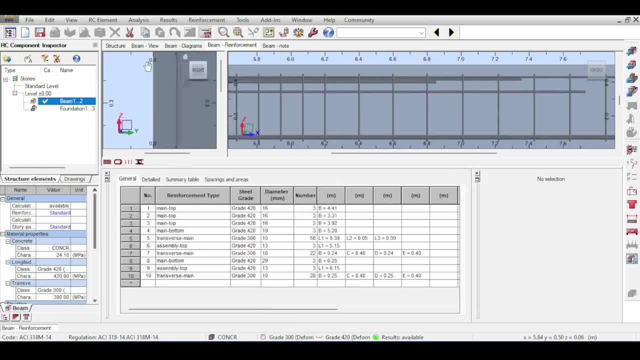 in real life, like i have less than this and i mean it doesn't look right, like those reinforcements don't seem to be right. so there is a lot of work to be done here and it needs some time. so the things i'm going to cover is not this, because this is like at the reinforcement. 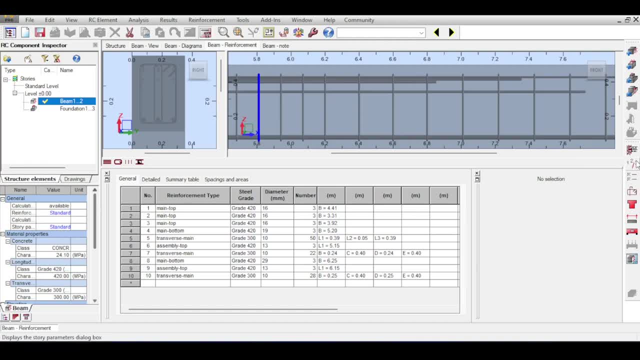 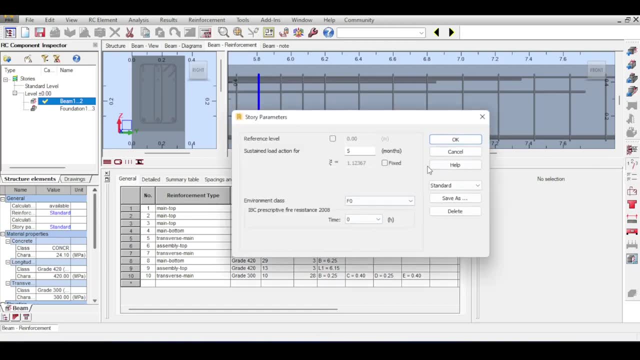 templates that you can change. i will actually go into the deep depths of the reinforcement itself. so the first thing you have here is story parameters, which has nothing to do with the error. the only thing that you can change here is the sustained load action four. this changes the long 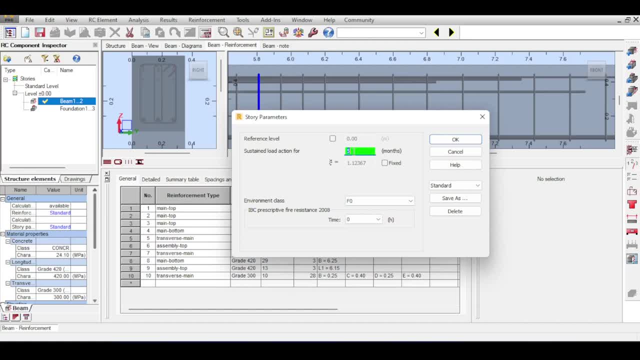 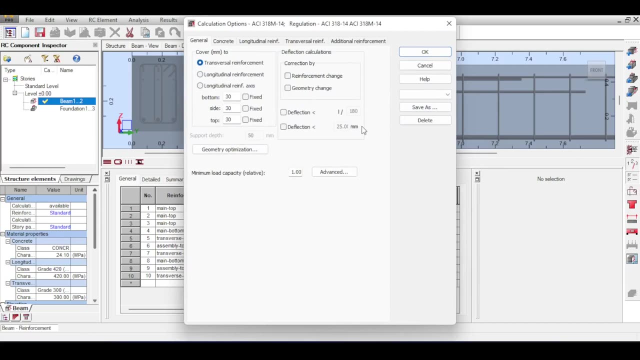 term deflection calculations because, according to the definition, the long term deflection calculations includes creep, and creep is measured after an x number of months. in this case it's five. now i don't care, because i'm using once again the ac recommendation for calculation options. this is where the fun starts now. first of all, for the first sign, here you have deflection. 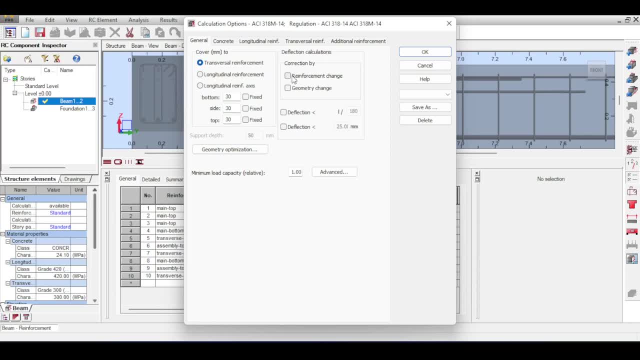 calculations and you can correct the deflection, ie solve the problem of deflections by changing either reinforcement or geometry. so i'm going to go into the geometry optimization section, optimization, and i'm going to touch this because, as we have agreed, i'm i am abiding by the aci recommendation section optimization geometry. 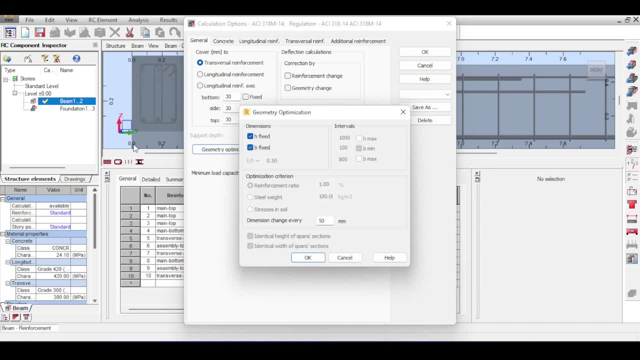 optimization may give provides robot with the ability to change your width and height because, remember, our width is 350 and the height is 500. you can actually allow robot to move those and change those heights to fit your design. i will not do that because usually the height of the beam is 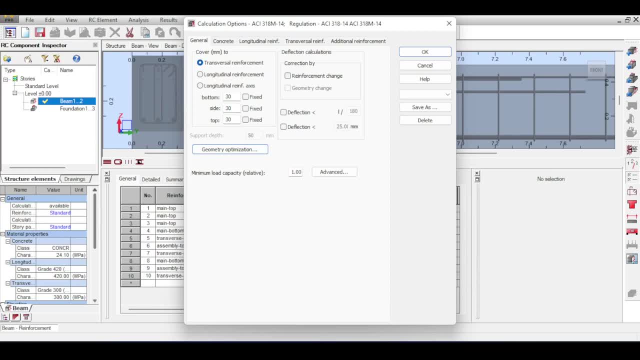 based on some architectural and other factors. so i rather let myself change the sections rather than the width and height of the beam, so that i can change the height of the beam, so that the beam is measured from the transversal reinforcement. that's perfectly fine. now, of course, the cover can be. 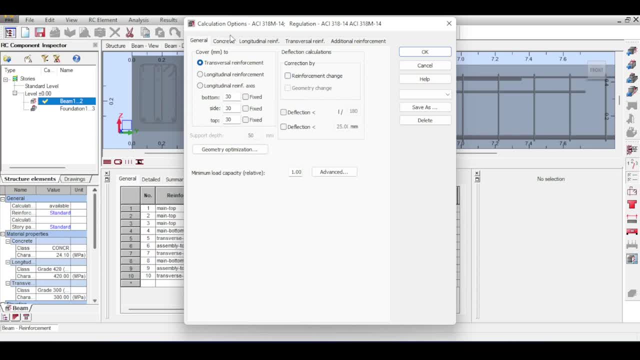 changed. you can fix your cover based on what the code requires from you. i will leave it as default like this for my concrete: i'm going to select me a concrete that is almost 30 megapascals. of course, you can switch any concrete you want. my concrete is not lightweight concrete, so there is no lambda. 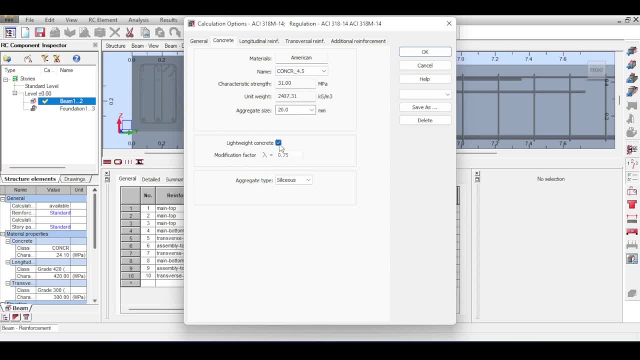 modification factor. if it's lightweight, you open it and change the lambda. this is provided by the aci code. also notice you can see in the title that those options are from the aci code and therefore you can see different things if you have different codes for longitudinal reinforcement, which means 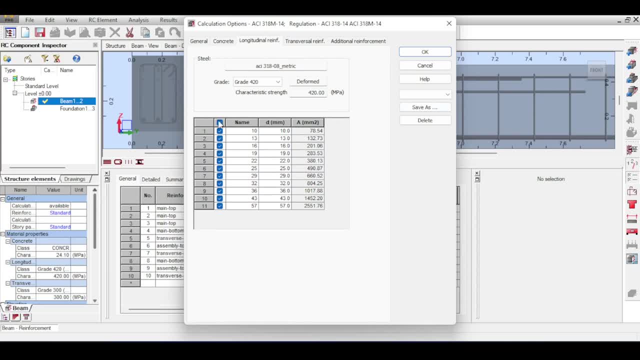 main reinforcement in the longitudinal direction. those are the bars that robot is going to use and this is the grade i will be using transverse reinforcement. now i like to use the same grade for both longitudinal and transverse reinforcement, so i'm using the 420 megapascal steel additional. 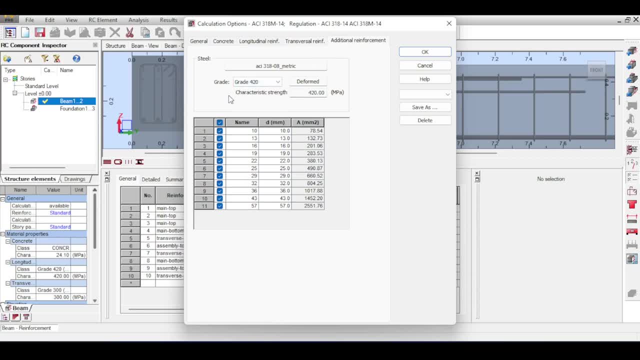 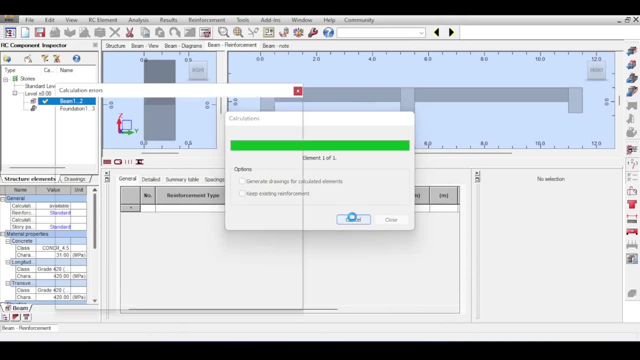 reinforcement, which is the construction reinforcement, is also 420 megapascals, so just click on. ok, now, if you run the analysis, the only thing that you need to do is to run the analysis, and that change is some reinforcement grading. but it will not work because if you click run, you can see. 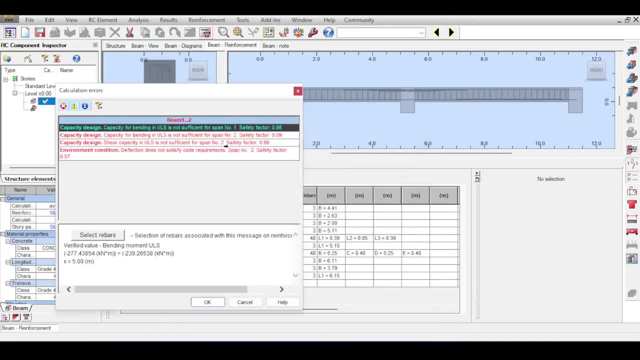 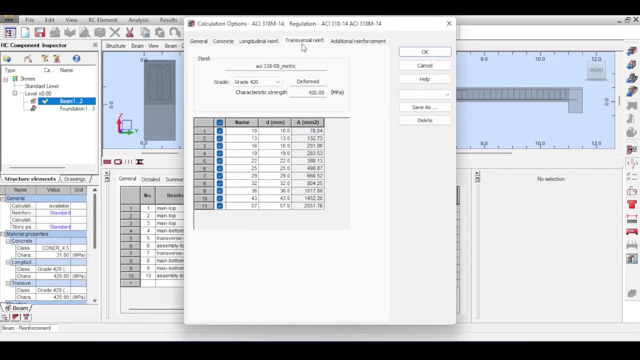 that, well, my arrows are not really getting better now. well, one of them seems to have disappeared, which is the shear capacity. i think it disappeared because i have increased the shear strength of my transverse reinforcement and this seems to have solved one of the problems. but well, it's not really. 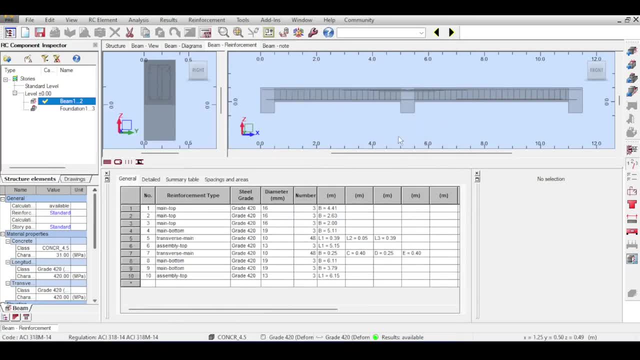 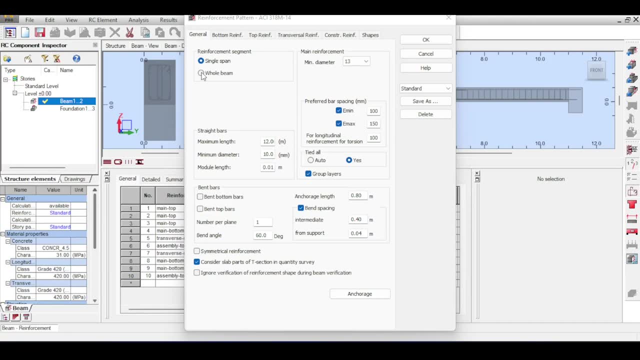 an effective solution, because i still have my three problems. however, we still have this to talk about, which is reinforcement pattern. so the first thing is that my reinforcement is not going to be the same as the other beam, so i will have it to be my whole beam, and the second thing is that i 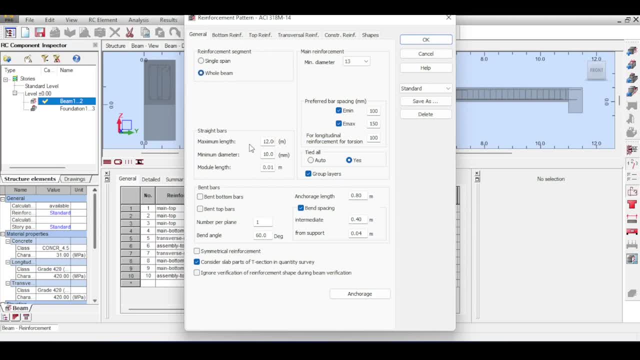 want my reinforcement to extend to the other span if it can, because each straight bar has a maximum length. so if it's possible to apply one bar for the entire beam, why not? so i will have it to be my whole beam. for the main reinforcement there is a minimum diameter of 30 millimeters, i don't care. 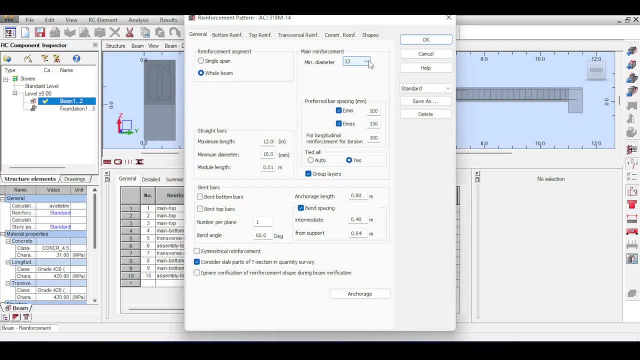 you can select anything you want, because robot will actually suggest a different diameter if it needs to do that. there is also the bar spacing: minimum, maximum and also spacing for longitudinal reinforcement for torsion. you can check that tight. all means that all the reinforcement in the cross sections have ties around it. well, this is not the case. i want it to be automatic, because 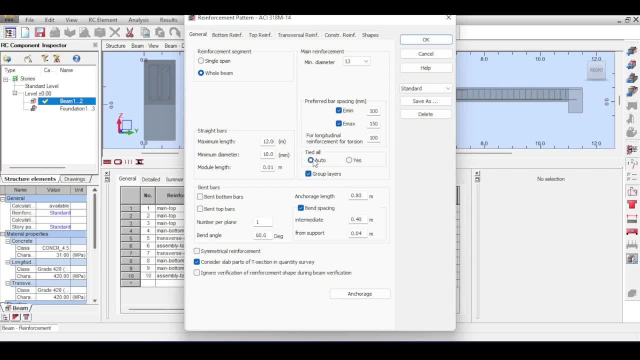 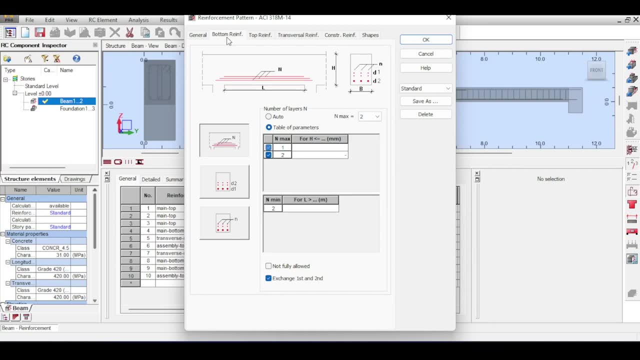 the asi code allows you to tie one bar and leave one other part untied if the distance between them is less than, i think, 15 centimeters or something, i don't remember. actually for bottom reinforcement. this is where the fun starts: you can control the number of layers, the diameter and the number of 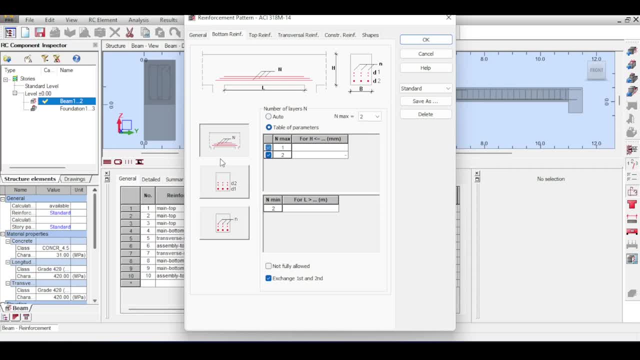 bars in an area. so first of all i will leave it as is. i will only increase the number of layers to four, just to allow it to increase the layers if need be. also, the layers are going to be determined automatically, which means robot will try one layer, two layer, three layer and four layers for top reinforcement. i don't want it to be as 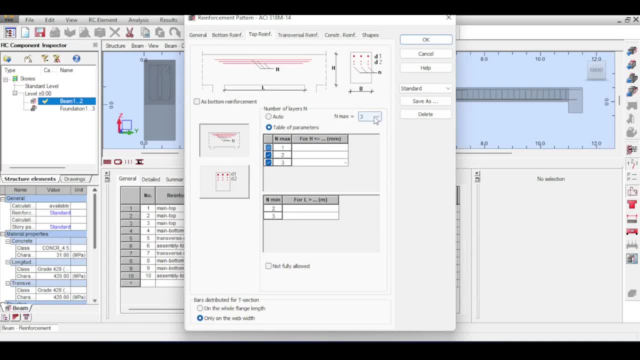 bottom reinforcement, because they are substantially different and i want my layers to be four, done automatically and you can see that there are diameters and there is a hidden problem here. you see, if you go to diameters- diameters- I'm not changing anything actually, but if you get the top reinforcement, you see that the 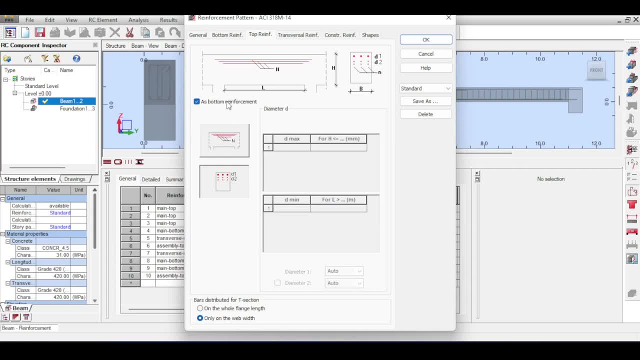 diameter is as bottom reinforcement. I don't want that, because usually the top moment is different than the bottom moment, so I think it makes sense that my diameters should be different. for transversal reinforcement I will keep it as is- I'll come back to it later- and for construction. 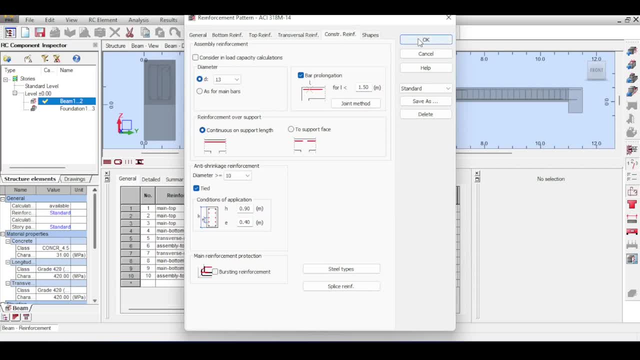 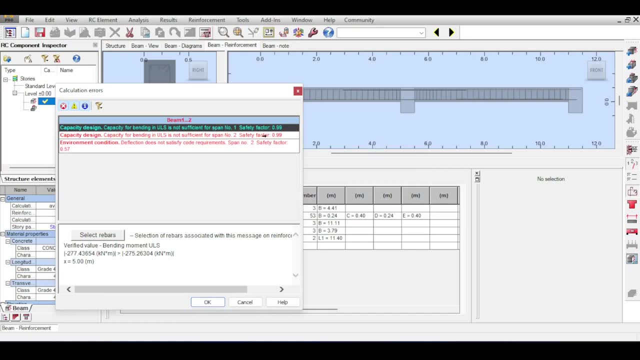 reinforcement. I will leave it as is. I'll come back to it later because I want to solve the problem step by step. so if I calculate now, it will not solve the problem. there seems one problem less and there seems it's almost solved- almost, but but not really so. if you go to the diagrams, you 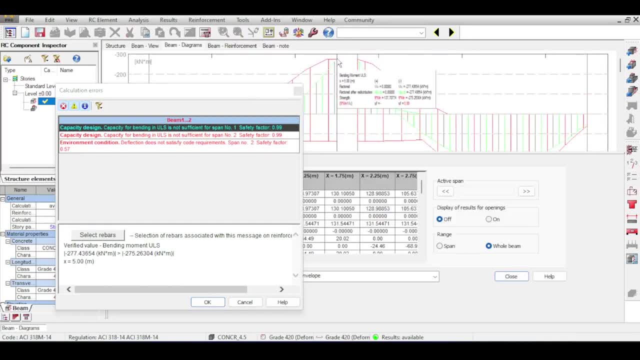 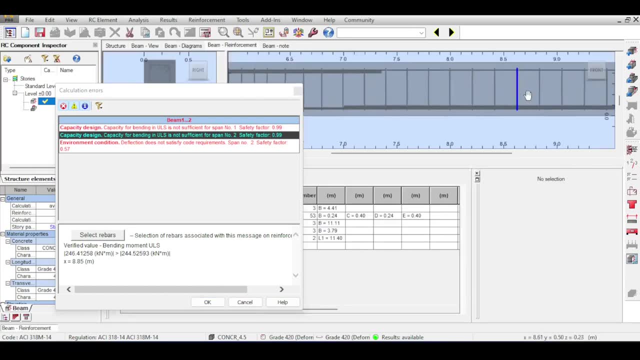 can see that it is almost so, but not really. here you have a one percent difference. it's really like it's really annoying, but well, it's not. it's not safe and if you go to your beam reinforcements and take a look, it seems that things look okayish. however, I have two problems. the first problem: I 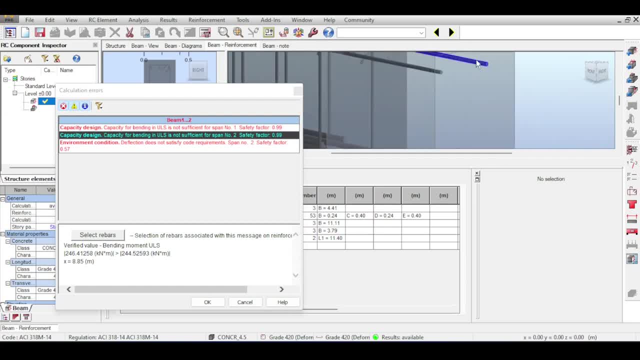 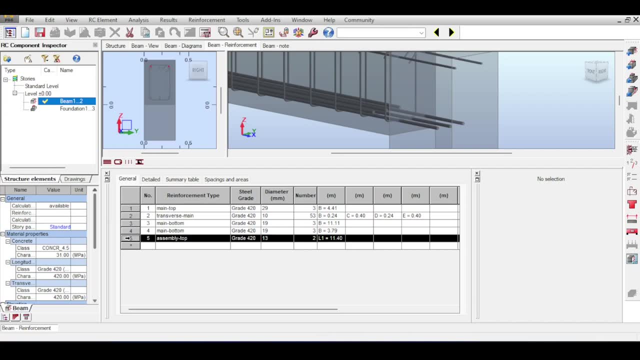 have with this reinforcement is this little tiny things. now, what are those? what's the meaning of this? what are those bars? those bars are actually called assembly reinforcement. if you click here, you can see that if you click on a bar, it will highlight you the bar. it's called. 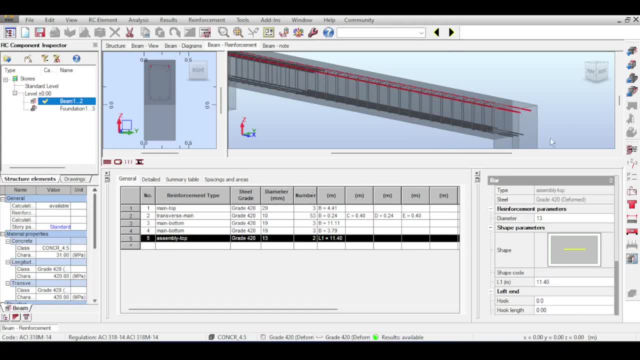 assembly reinforcement and you have assembly reinforcement in top and assembly reinforcement in bottom, if need be. there's a strange thing about assembly reinforcement. the strange thing about assembly reinforcements is that this reinforcement is not is by default not taking into account when calculating the strength of the beam, which is a shame because I mean it's. 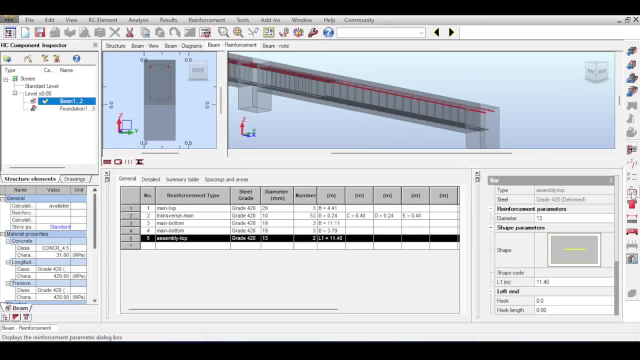 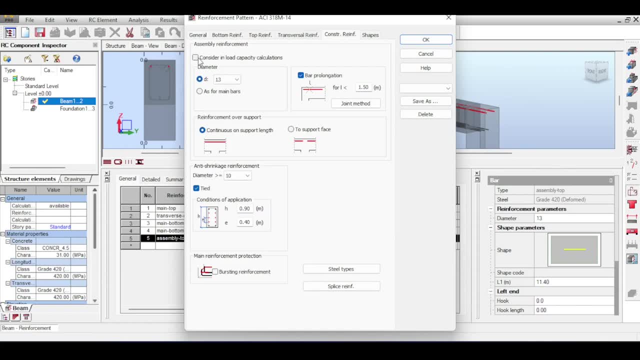 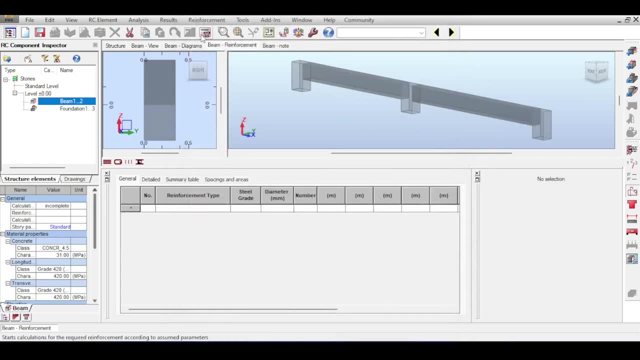 there. why not use it so to change that? you can go to once again reinforcement pattern, to the construction reinforcement which is called assembly. by the way, you can see that you can actually click on. consider the assembly reinforcement in load capacity calculations. so that's fine. if you click on that it will work. but there are still more improvements to be done now. 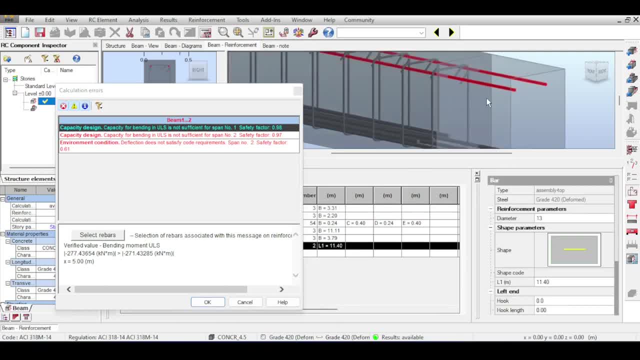 the assembly reinforcement now is used in the strength calculation and that's why suddenly the main reinforcement that was here disappeared. so okay, it seems to make sense to use the assembly reinforcement, because- why not? it's there now. the second thing is that it seems my assembly reinforcement is really small in. 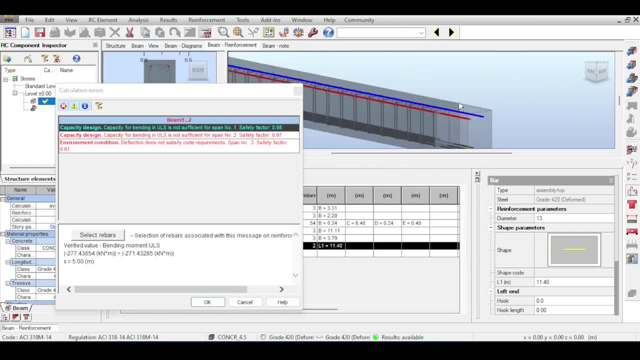 comparison with my main reinforcement. and this creates practical problems because usually you like to have your at least your top reinforcement alone to be at least of the same size and the bottom reinforcement alone to be at least of same size. if you can now this size variation would. 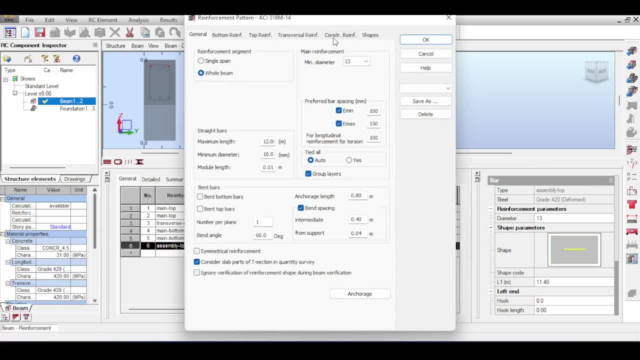 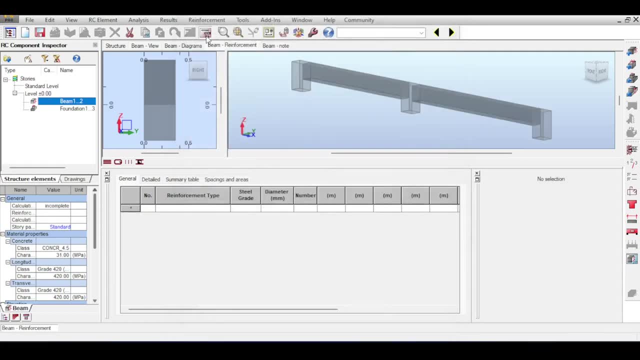 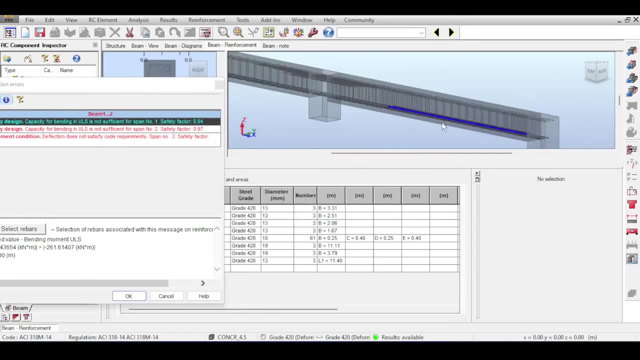 cause practical problems. so actually i can change this by going to construction reinforcement and clicking on like the diameter is as for main bars. so now my assembly reinforcement is going to have the same diameter as my main reinforcement and you can see that well, it starts producing meaningful drawings. but i mean, look at this, this is like. this is too much. this steel is. 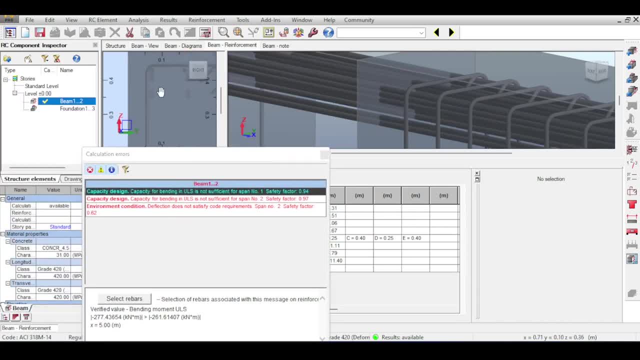 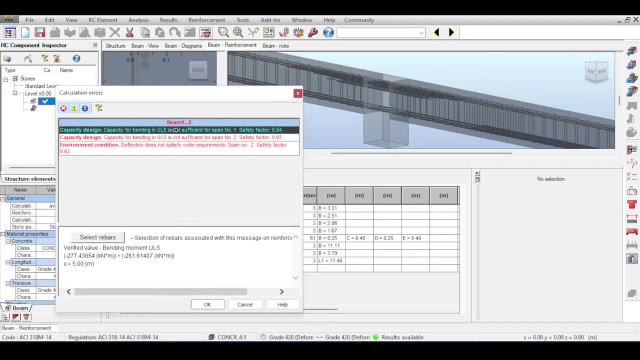 i don't know how we even can cast this. this is not practical. i will take a look here. this is too much so there are still problems and i'm solving it step by step. so the capacity in the bending is still not sufficient. and there is one last trick why this is the case. so allow me to show you this. so if you go to 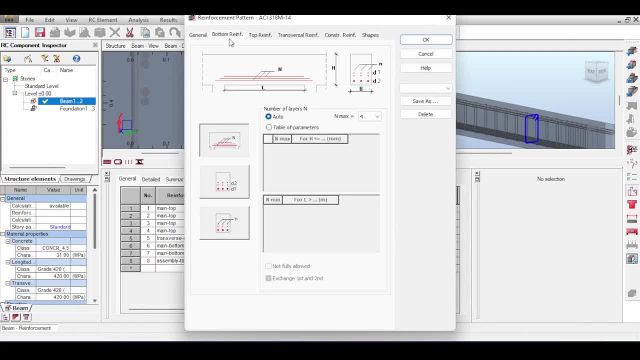 reinforcement pattern. now go to bottom reinforcement, go to the number. here you can see that the number is between two and eight, and robot tries to match the number of the bottom reinforcement with the number of top reinforcement, which is something i don't like. so i first of all change. 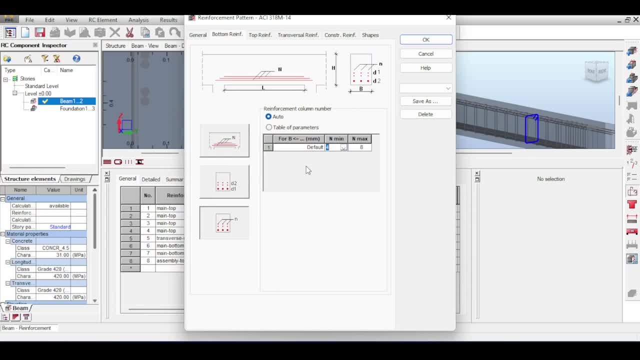 the minimum number of bars to four to have a two-fold effect. the first effect is i want to reduce the size of the bar. the second effect is i want to allow robot to have more bars on the top. so if i click on that now and calculate, 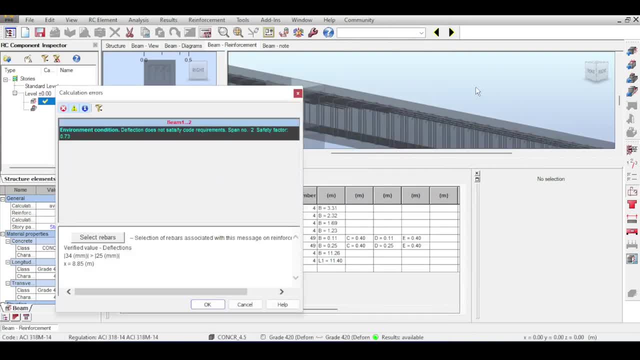 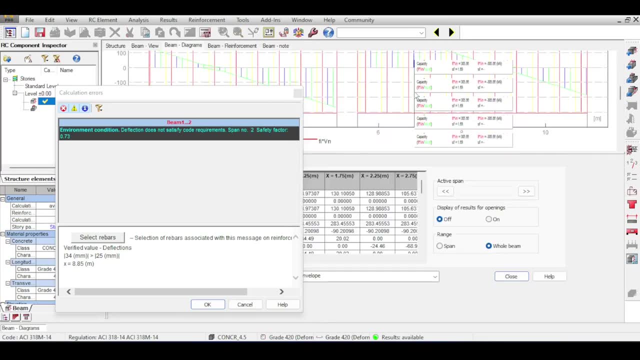 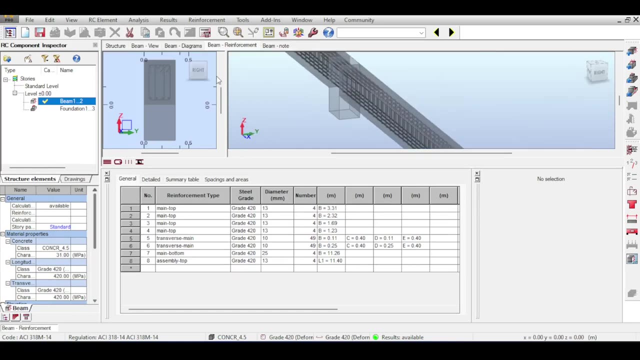 you see, well, everything seems to be working perfectly, because now i have no problems. if you go to beam diagrams, you can see that everything is working in perfect order. so yeah, i have just accomplished my design. but i mean, i'm a perfectionist, so there is still a problem. 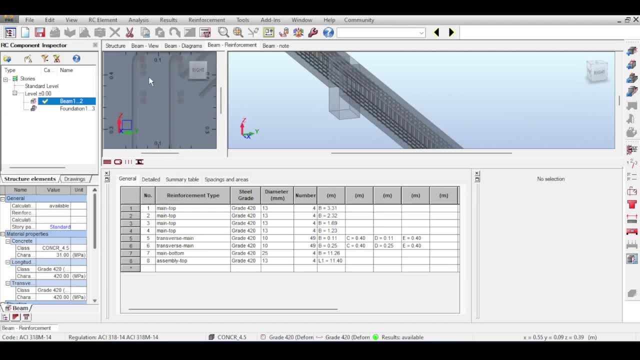 uh, well, okay, the bars seem to be okayish, i don't know. there are too many bars like i don't know. maybe i should decrease and affect the number of bars. more than one bar should, for example, i'll try to get a few bars lower than a smaller one to away. 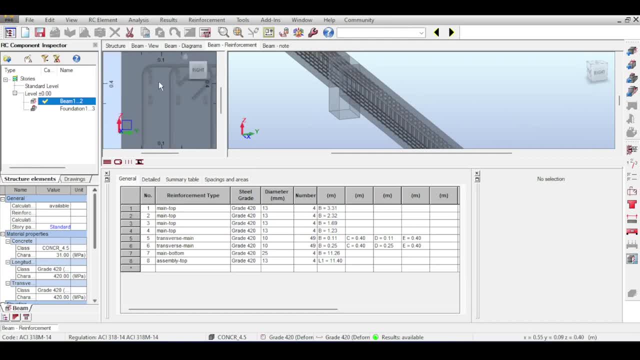 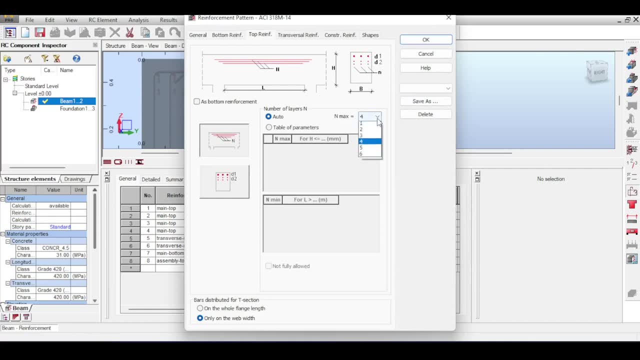 number of layers, because now I'm doing only improvements to this. so I think number of layers is too much. I'll just change that. so I'll just go to reinforcement patterns, one again, go to my top reinforcement and just make three layers, for example, and just hit OK and try again. so see, this is some sort of. 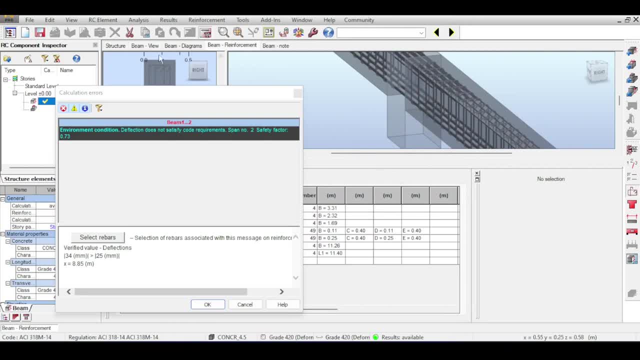 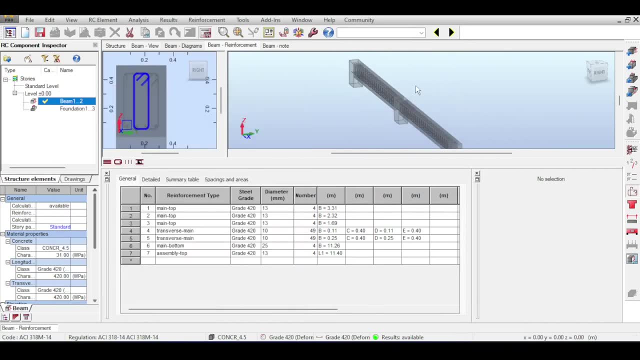 repetitive task that you will have to keep continue doing until you finally get this. now you have three layers and robot actually increase the bar size to match those layers. now- I will leave this for you to investigate- you can actually even change the diameter of the bars. I mean, look, the top is 30 millimeters in. 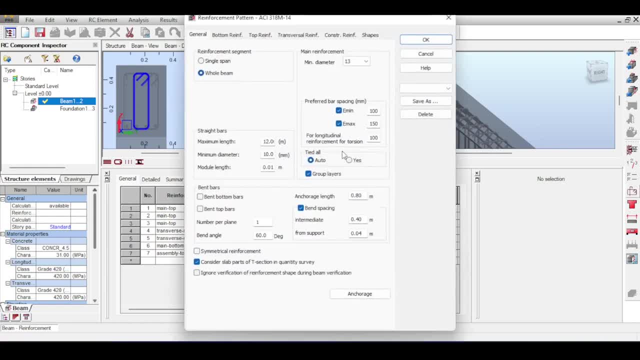 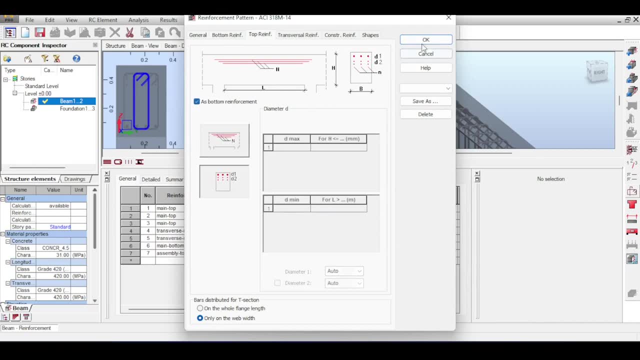 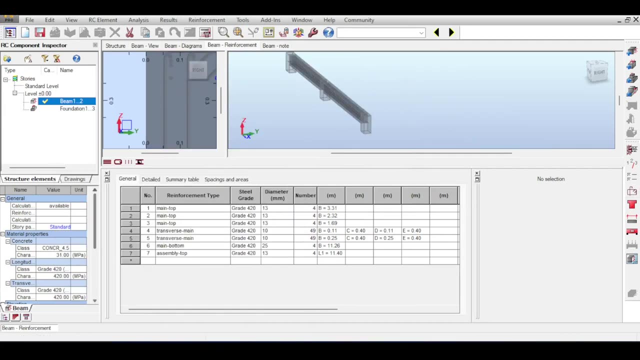 the bottom is 25. I mean you can actually unify the diameters. if you want so to bottom reinforcement to diameter, I can match it to become as bottom reinforcement. I just click on. ok, maybe this would be better now. you see, I'm just doing some minor improvements. the best way of learning those things are: 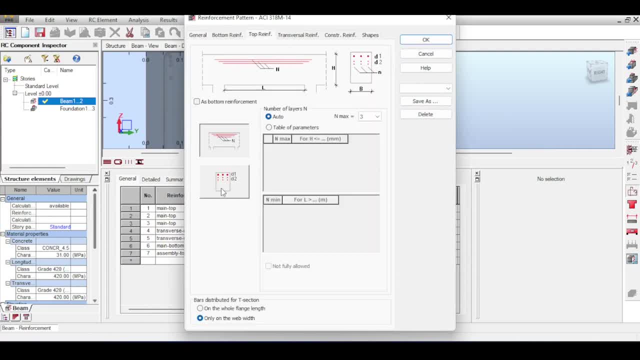 just to keep you know, changing stuff and getting a feeling of what those things are doing, what are the effect of those things? you can even force robot to use 25 millimeters and run the analysis. and now it's 25 millimeters everywhere. and now, I think, 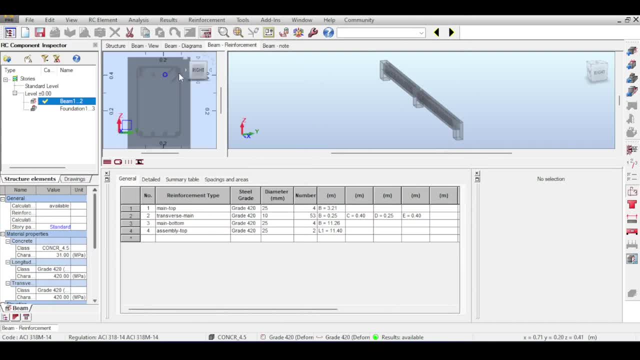 now. I like it because now it's only one, one layer of steel bars, all right. so I mean you can play around and I think I have reached a beam that I kind of like, but there is one problem left. the problem that I have now is with stirrups. 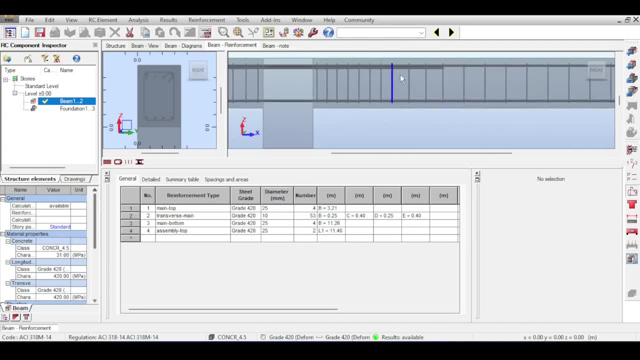 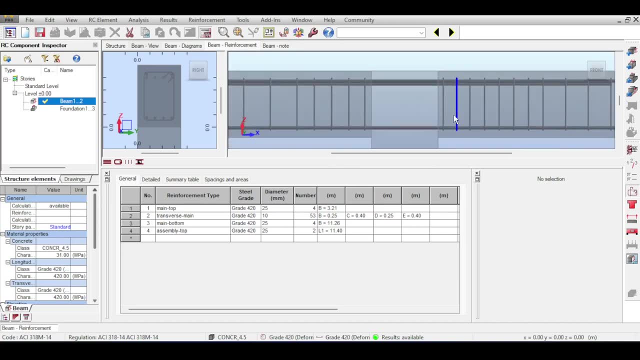 it seems that like, look, here you have a spacing, here you have a different spacing, here you have a different spacing. I mean, this is nice and dandy, but it seems that my setup spacing is not even to the closest five centimeters, which causes practical problems. trust me, I have seen a lot of setups that cause confusion among the 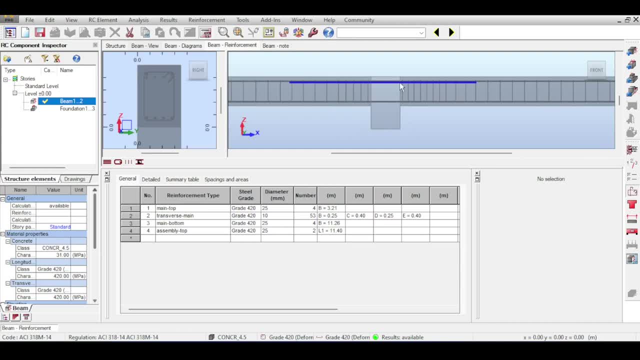 workers. so usually I- and this is a personal opinion- I usually like my startups to be five centimeters spaced, like 50 millimeters, 100 millimeters, 150mm and so on. so I will change that. now, how do I change my transverse reinforcement design? well, I got reinforcement pattern to my transversal reinforcement and I 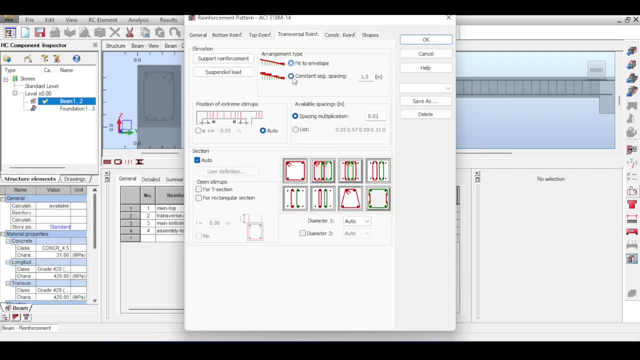 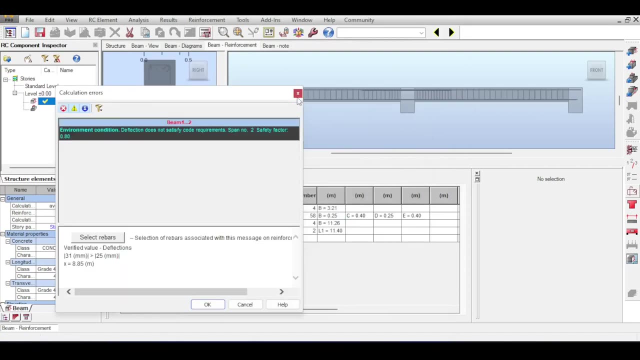 don't want it to follow the envelope exactly. I wanted to like just design each one meter segment alone and I want my spacing to be to the closest five centimeters. now this might break my analysis, I don't know really. I just try this right now, hit the okay button, analyze again. so I hope that my beam yeah. 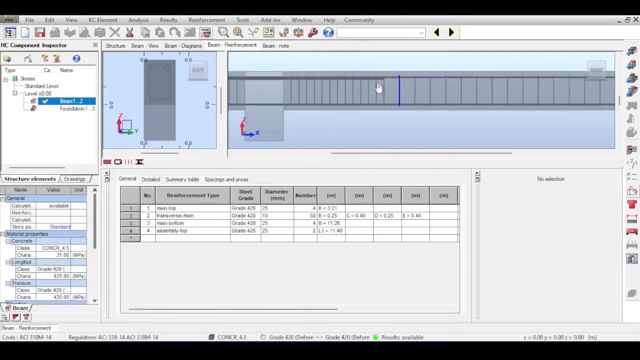 it's works perfectly. now those are. you can see that there are just two spacings. there is one spacing, it seems it's five centimeters or ten, I'm not really sure- and the other one is 20, it seems. so, yeah, now I am happy and I think my beam is perfectly designed. I can 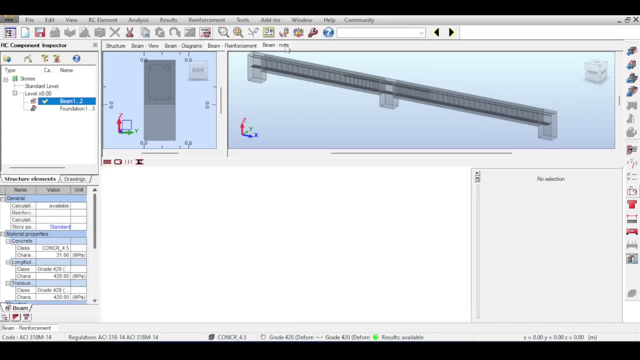 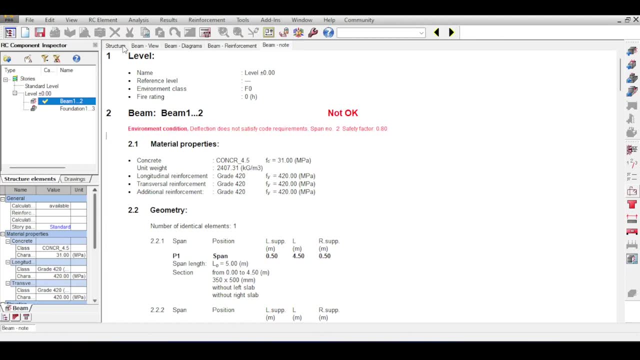 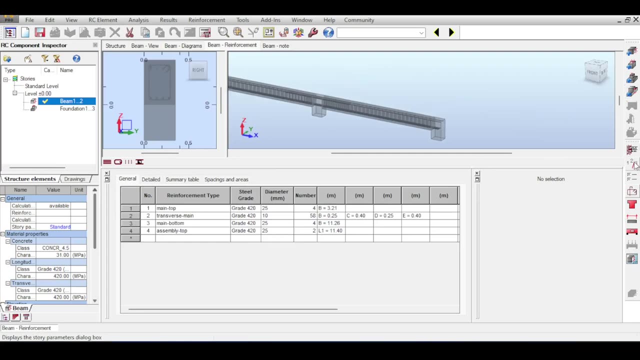 start looking at my calculation sheet and export me some drawings. if you go to beam note now, it will still tell you: not okay, because of the deflection. but nobody cares, I can quickly hack that. I will hack that because I told you that I am conforming with the ACI code, which allows me not to check any deflection if 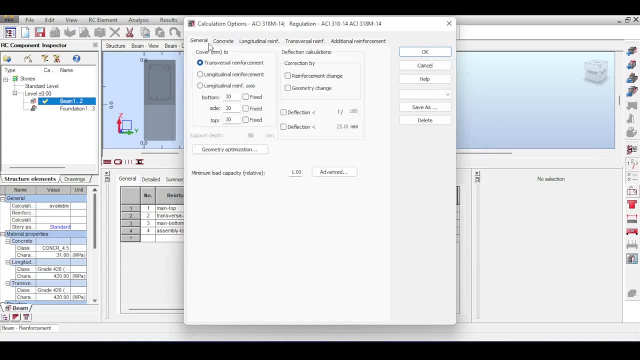 I abide by the minimum value of the deflection if I abide by the minimum value of the deflection from my beam height. so I just go to my general here and just tell him: hey, listen, man, I don't care what your deflection is, even if it's 100. 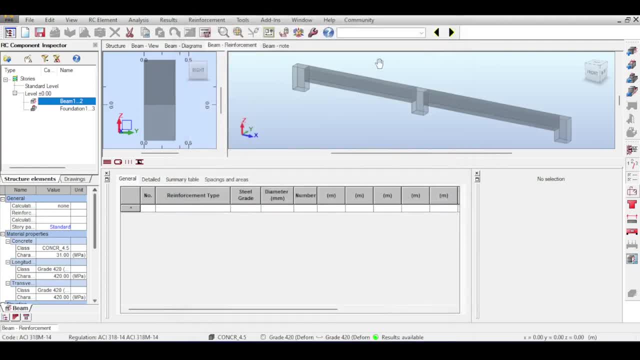 millimeters. I don't care, because I'm abiding by the ACI code recommendations. so now, no errors, I'm just I. this is a hack, by the way, that's not a solution. so if you go to review note and we see that the section is okay. 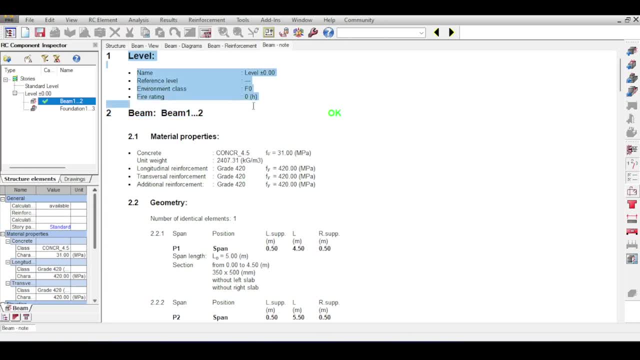 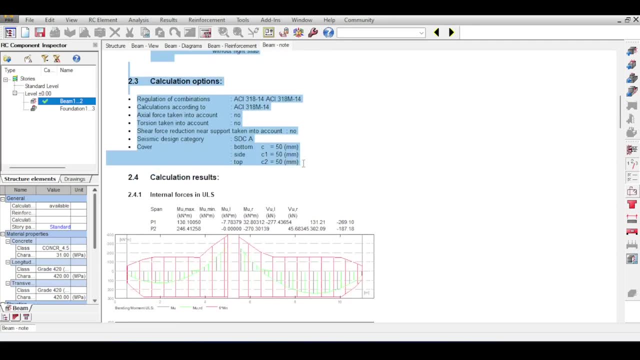 how can you read this? well, it tells you some information about the beam itself, about the material used, about the spans and about the calculation options you're choosing, and also the reconstruction鬚. now, the cover is 50 millimeters, depending on the code you can force it. 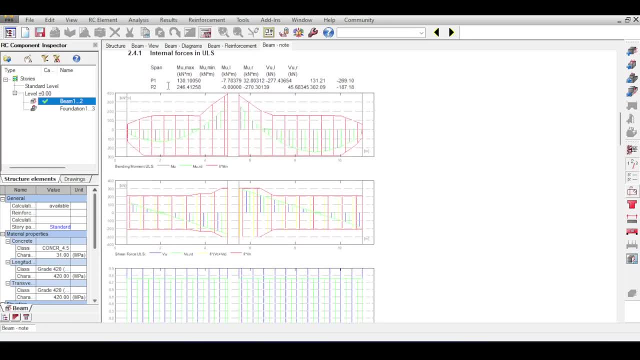 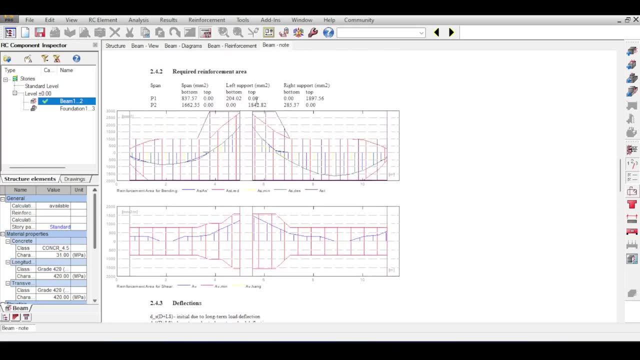 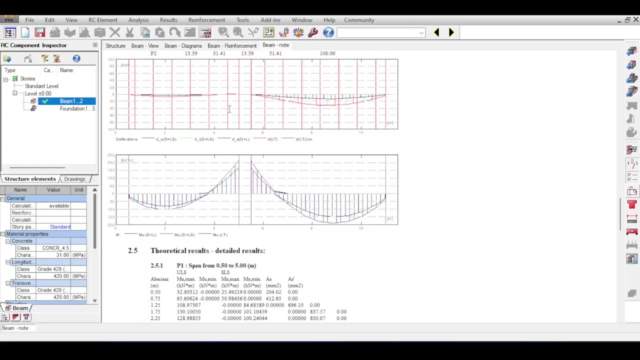 to change. if you want, I will leave it as is. you can see that the internal forces are being covered perfectly by the reinforcement and that satisfies also the enforcement requirement which is required enforcement. and finally- I just skip too much- you can even see that the beam is calculated by different points. 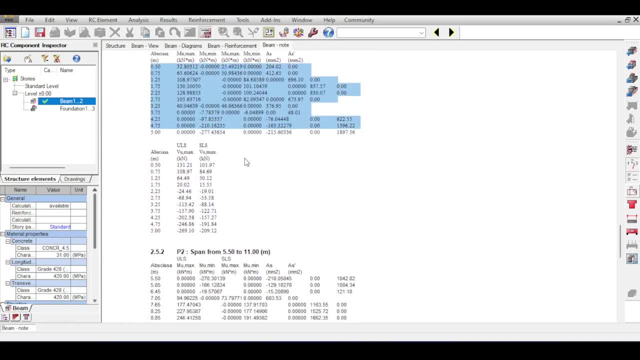 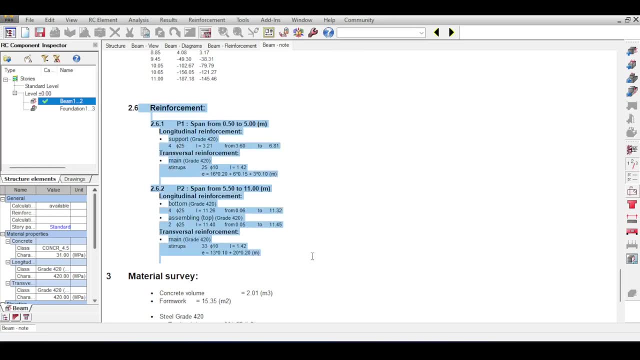 and it shows you that, for all those points, the reinforcements are able to carry the required forces. finally, and this is really important, you get a quantity surveying, and this is what I love in Autodesk robot. it gives you a quantity survey of what you need and this is basically what you will use to 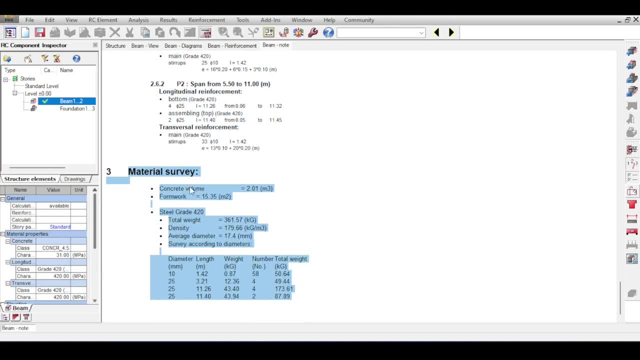 buy the stuff you need. so you see that for concrete it's two cubic meters. the formwork, which is the side area, is 15.35 meter square. they still required. the total weight is 361. now, the density is something I really love and like because 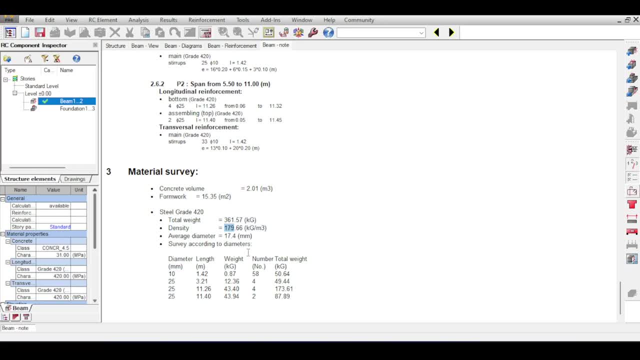 usually I use this. you can see that the density is something I really love and like because usually I use this in estimating the required steel. now, this has nothing to do with Autodesk robot, but whenever I work on contracts you see that in quantity bill of quantities in. 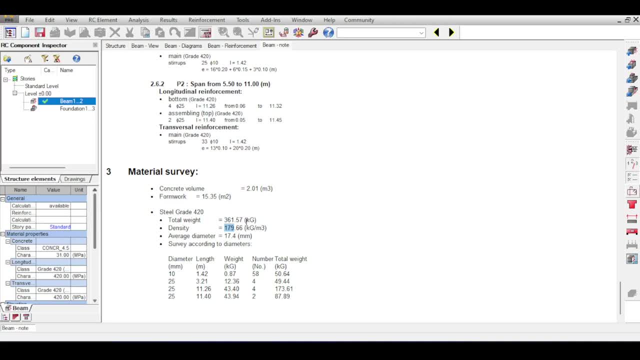 those contracts it tells you to like basically provide I don't know, like 30 cubic meters of reinforced concrete for beams and it never tells you how much steel you have in those beams. now, usually I know that for beams your steel is between 150 and 250 kilograms per meter cube. so I see that this is. 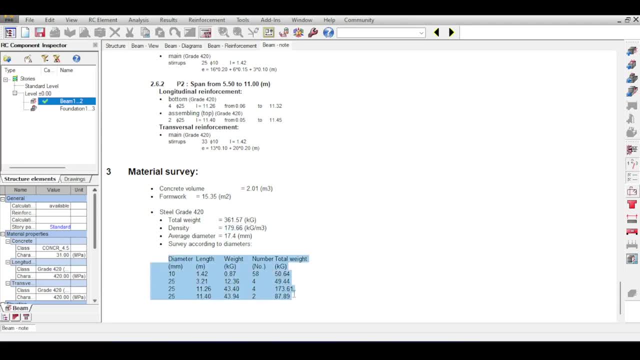 perfectly fine and you can see that you have a list of shopping, or a shopping list, basically, which gives you a fine diameter, it gives you the length, it gives you a number of pieces and the total weight. allow me to give you some practical advice here. this: those lengths are produced by the machine. 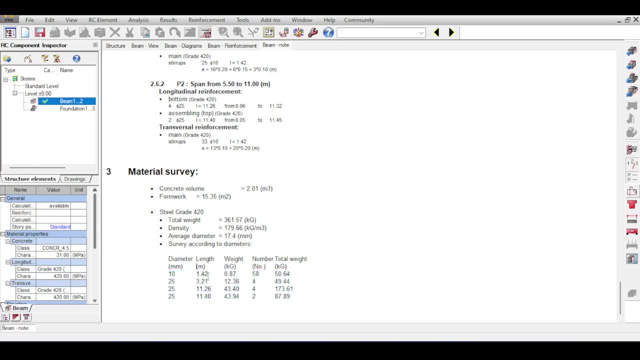 which gives you some strange 1.42 meter steel bar length. now, depending on the country where I were working- some countries, every centimeter is perfectly fine, like you can ask. you can ask a steel manufacturer to provide you with a steel bar of one point three, three, three meters, if you want. now, this is a 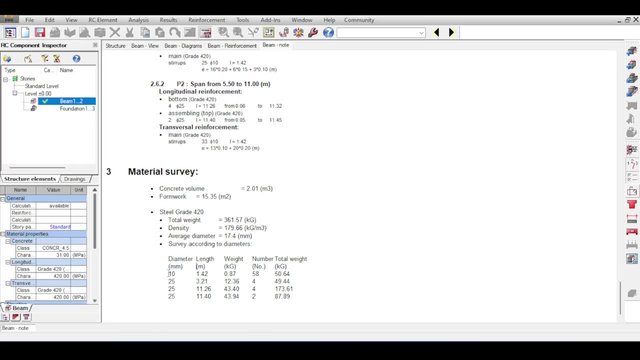 simple example of a steel bar length. in some countries- I don't know in the countries where I worked- usually steel is cut into lengths that make sense, like one meter, 1.5, 2 meter, 3 meter, 4 meter, and the criteria here is that you cut. 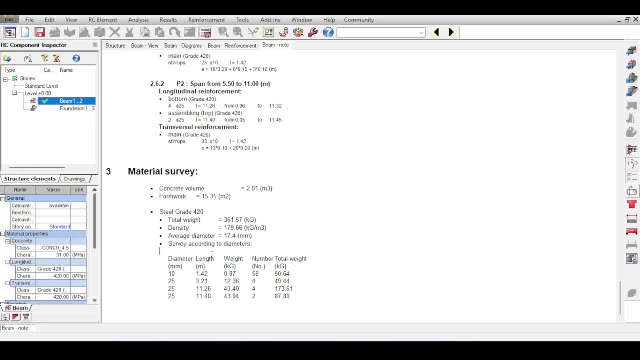 your steel bar into lengths that are able to be divided, meaning, if your steel bar is 12 meters from the manufacturer, you should divide it into pieces that are able to be cut without any excess. for example, if you choose to cut your steel bars to 5 meters, if you have a 12 meter bar, which this means that you can. 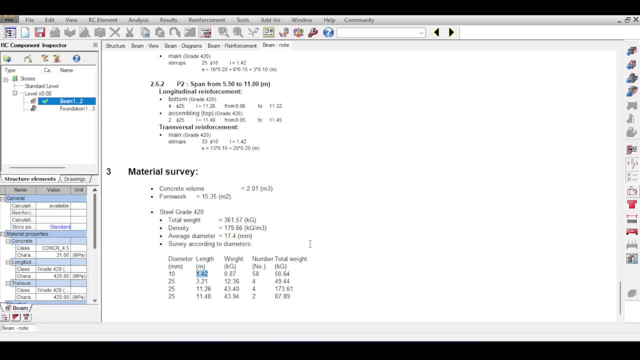 only produce two pieces 5 meters from your 12 meter bar and you will have an excess of 2 meters and you need to think where you should put those 2 meters to avoid any loss of steel. this gets doubly important if you have excesses less than. 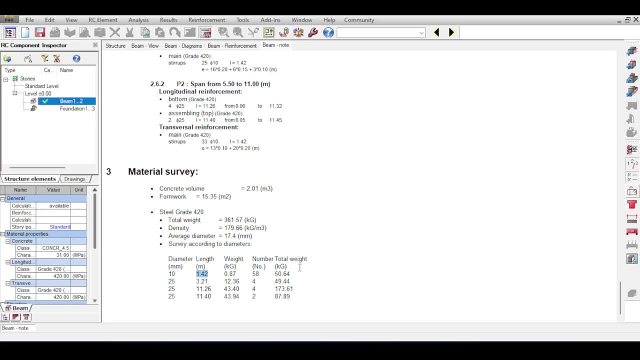 1 meter, because it becomes really hard to use this excess anywhere, so it becomes a waste. what I'm trying to say here is that, as a designer, you should always double check your lengths before you provide any tables and modify them to make more sense of this. speaking of tables and drawings, well, you can. 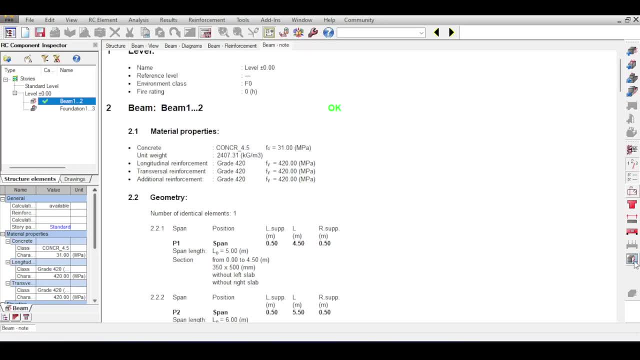 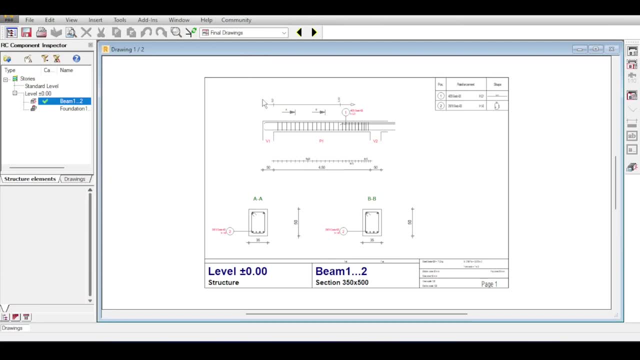 actually produce some drawings by clicking on the drawing button. if you click on this button here, if you click on that, you can start seeing the drawings of your beam. of course, this is not the full beam. this is only one span and you can select the next span and the previous span from those two arrows and 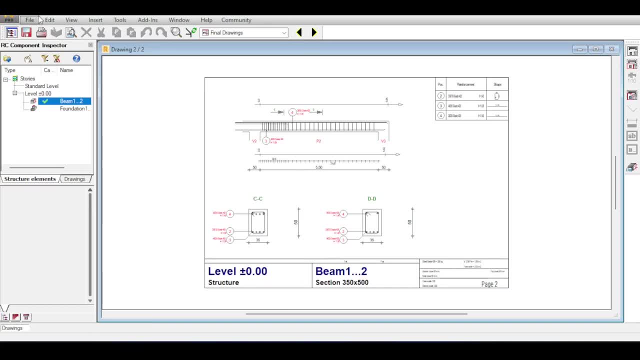 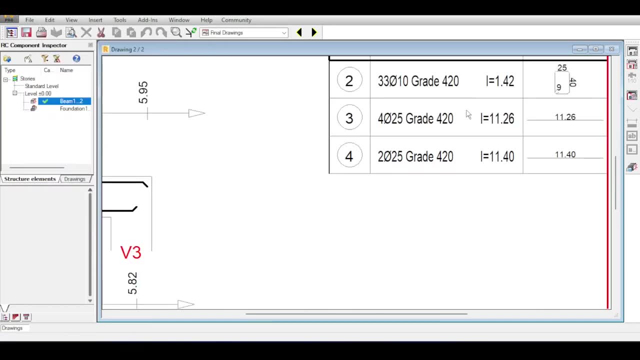 it seems everything to be fine. you can all can, of course, click, find and export this, or save it in a different format and export it as DXF or your AutoCAD, and you can see. this is really nice. it tells you each bar with a number and tells you what the length of the bars is. now, here is where your human 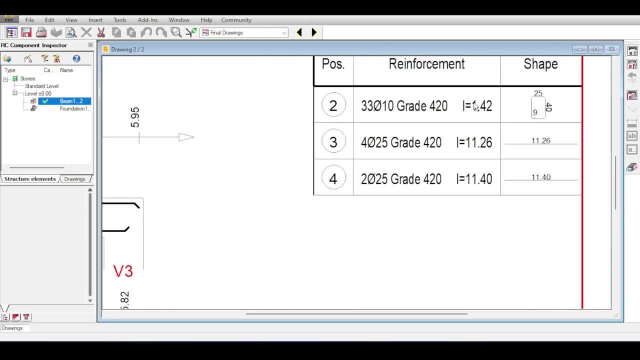 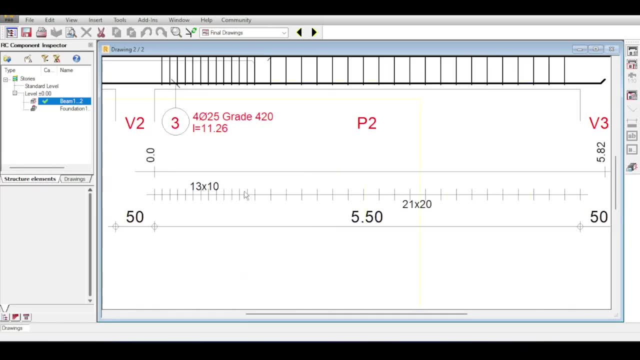 intervention is required because sometimes the bars length doesn't make sense, so you would add a little bit length to it to make sure that it does make sense. you can see also that the stirrups are here placed. the first stirrups are at 10 centimeters. seems that the units here are in centimeters. I'm 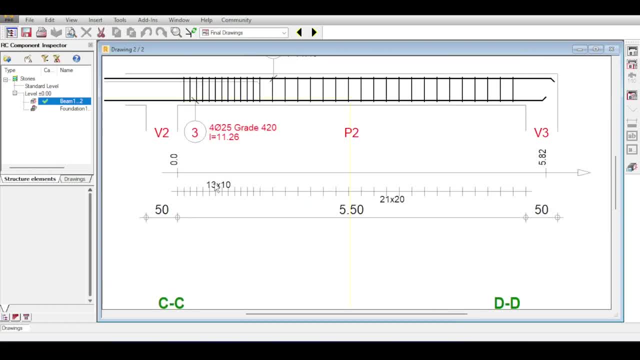 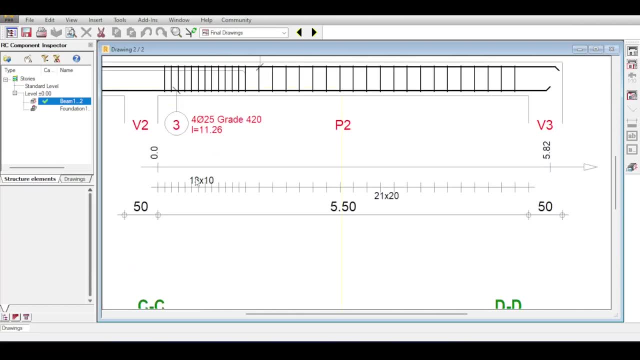 surprised. I think I spoke. I think I have asked it to be in meters, but it seems that those units are in centimeters. I really don't know why. I think I would check out why this is the case. anyway, you have 13 stirrups at 10 centimeters and 21 stirrups at 20 centimeters. you 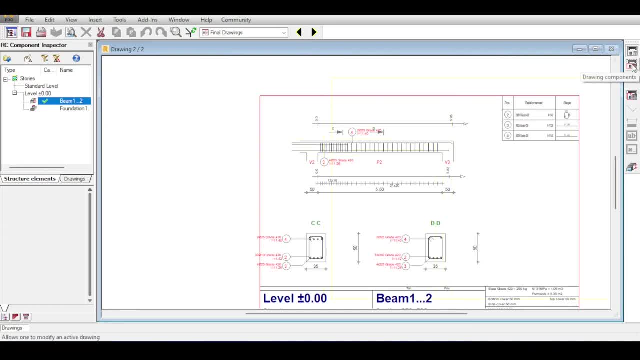 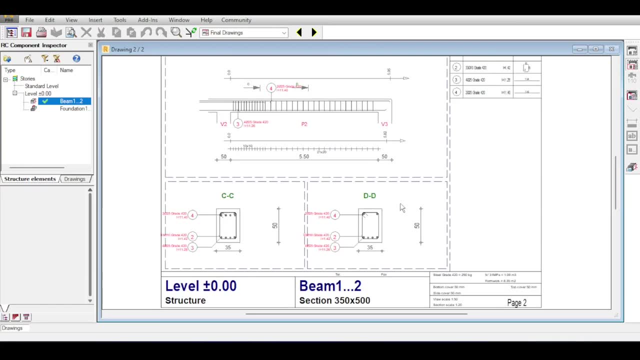 can actually modify this by clicking on this button, which is drawing components. now you can click on any component and modify it. so, for example, this DD section is taken here. if you click on that DD section, you can actually choose where this section is taken. so if you click on this section, you can actually 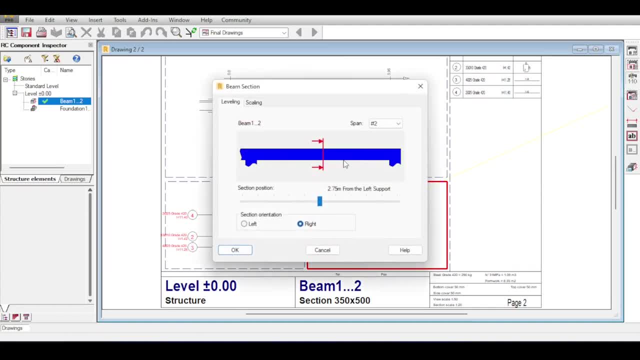 choose where this section is taken. so if you click here, which is called section location and scale, you can move the section DD from any position you want, for example here, and you can change the scale if you want. you can add a different scale if you want. I just leave it as is, but I'll just move my section. 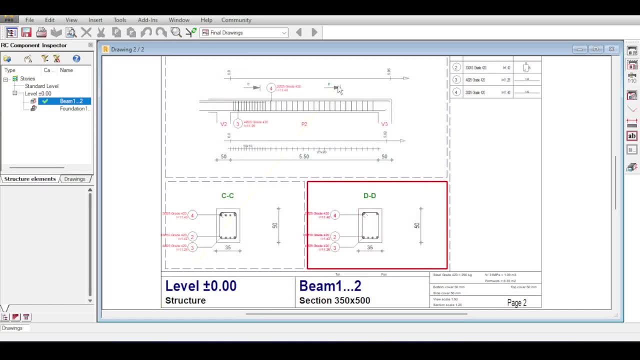 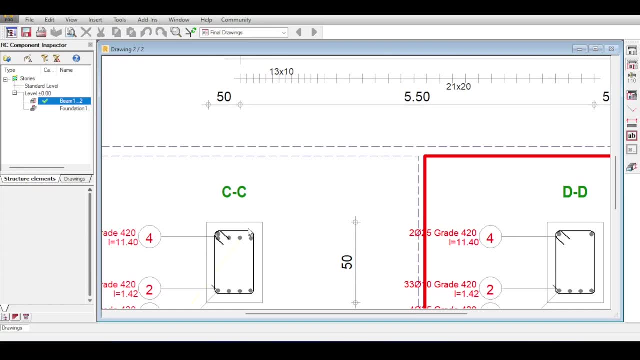 here. if you click on OK, you can see that DD has been changed and that the section is now here. this CC section, it's taking perfectly, because you see all the bars. I mean, yeah, those are a lot of options you can play with and that's it, that's. 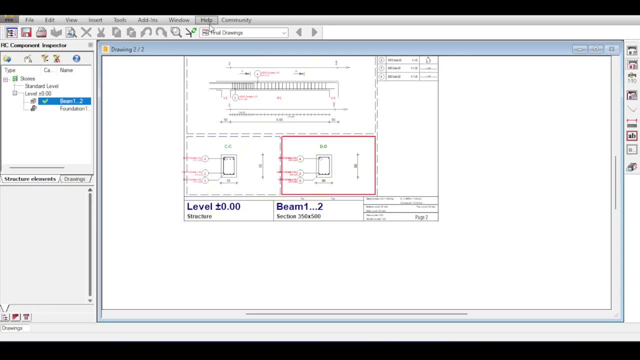 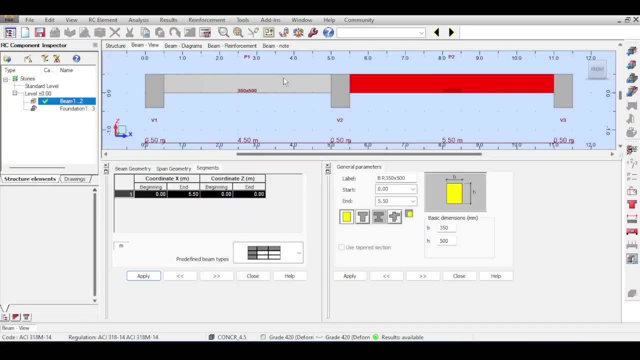 everything I wanted to talk about in this video. so thank you for watching and I'll see you in the next video. bye, bye, bye about today. this is how robot provides reinforcement. it's really a nifty and nice tool and there are a lot of options to be studied. here. I just tried to go. 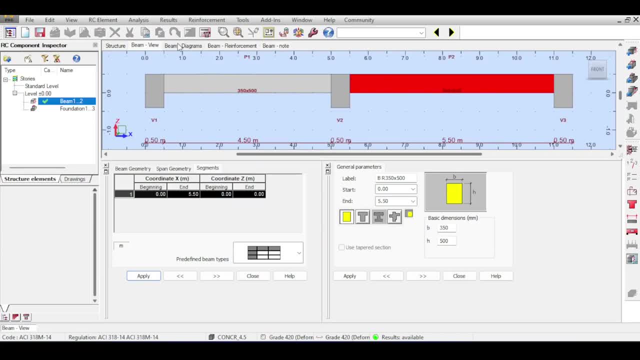 through the process step by step, and eliminate all the problems I have seen during this process. that's all what I wanted to explain this time. if you like this video, I hope that you share this with you. subscribe to the channel like comment of the liking. it helps a lot, especially subscribing, because it 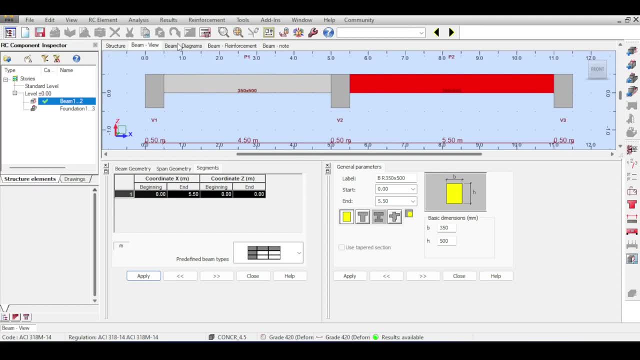 increases the reach of my channel, which is something I really appreciate. and, as usual, if you have any questions, please feel free to ask me in the comments below. any questions, you can always post them in the comments. this is the civil engineering essential channel and we will catch you in the next video. 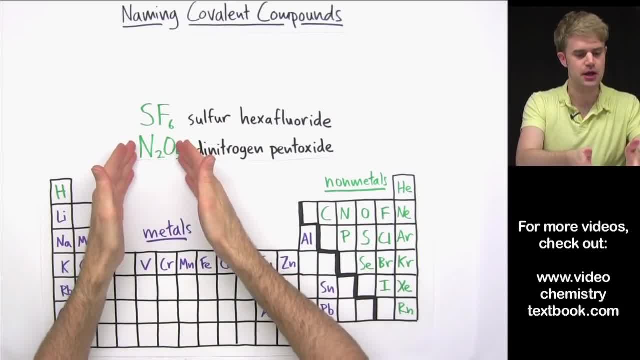 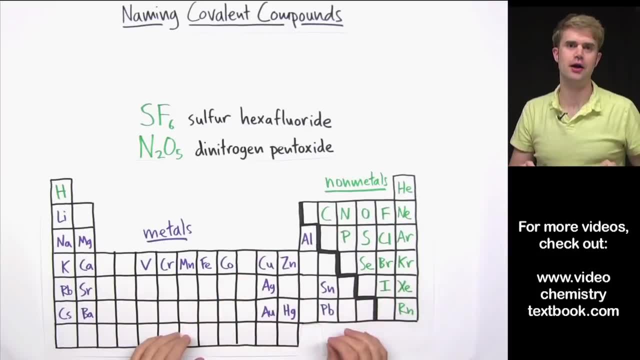 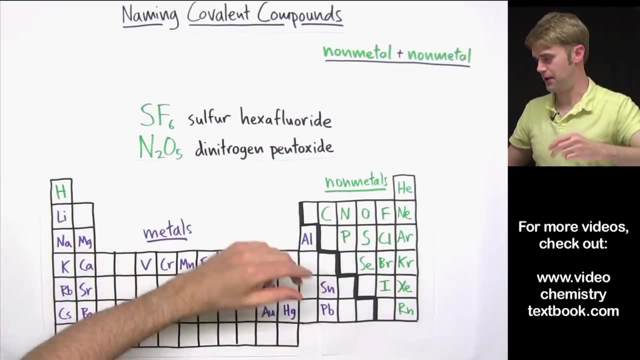 Let's look at how to write names for compounds like these that are made of two nonmetals. The nonmetals are the elements to the right of the staircase on the periodic table. Now, compounds like these that are made of a nonmetal and another nonmetal- two nonmetals- are called.